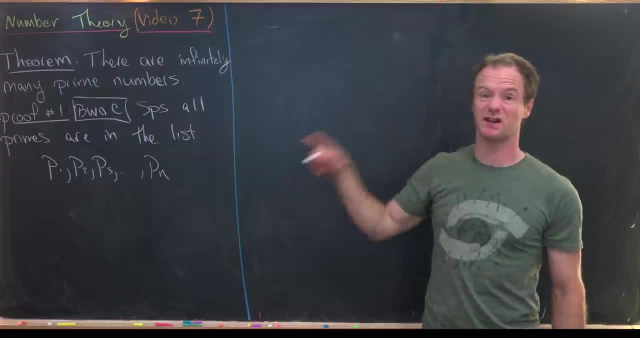 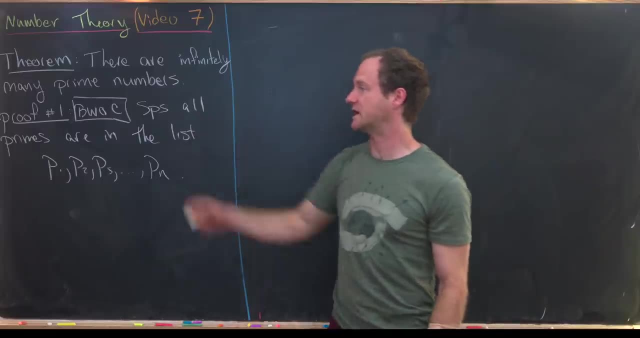 So here we've got n primes. This is a little n Okay. so next we're going to form a very like important number in terms of getting towards our contradiction, and that number will be the first one. So we're going to start with a very like important number in terms of getting. 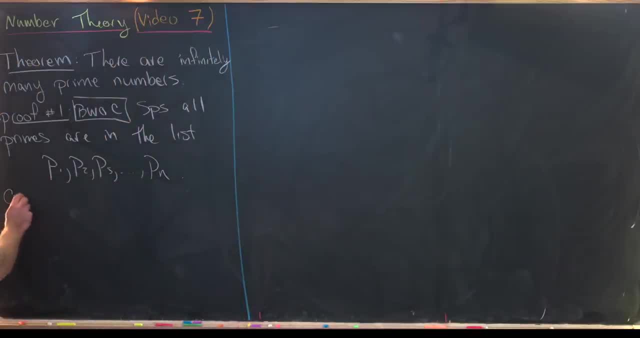 towards our contradiction, and that number will be the first one. So we're going to start with a product of all of these primes plus one. So let's consider capital N, which is equal to this product, p1,, p2, all the way up to pn plus one, And I want to notice the following. So this is a. 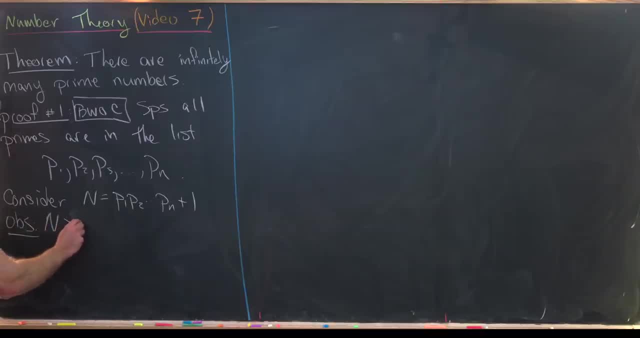 pretty easy observation, and that is: capital N is strictly bigger than pi, and this is going to be true for all i between 1 and 2.. So this is a pretty easy observation, and that is capital N and n. Well, why is that? Well notice, it's the product of all of these things plus one. So 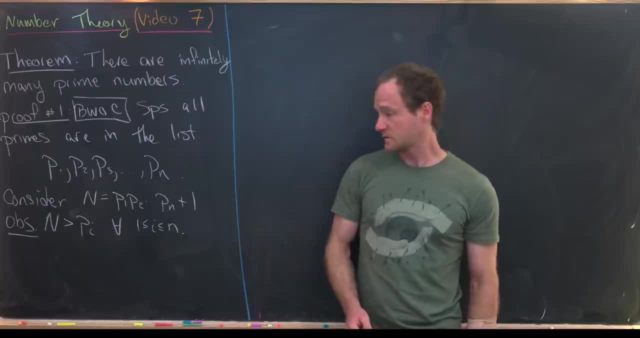 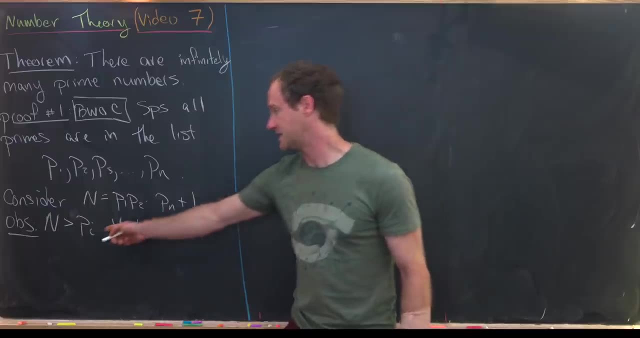 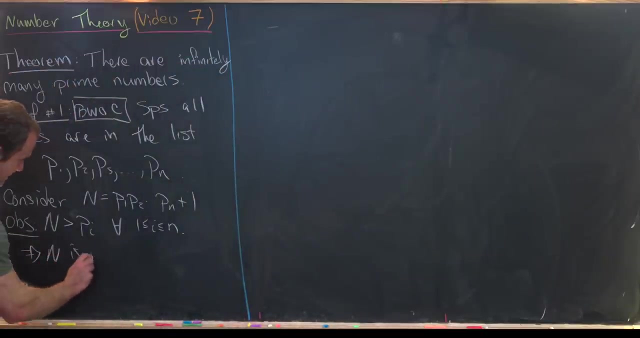 that's pretty clear. Okay, so that means that this capital, N, cannot be on this list. Well, why not? Because it's bigger than everything on this list. So in other words, we know that n is not prime Great. 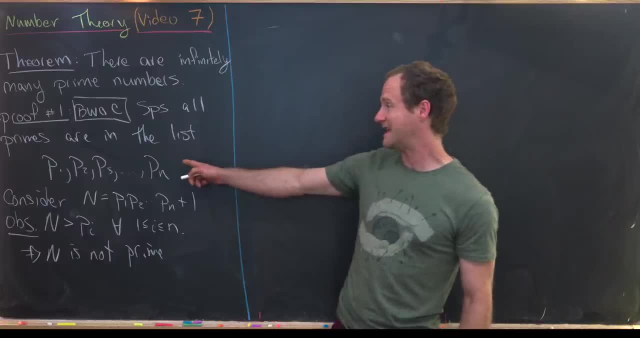 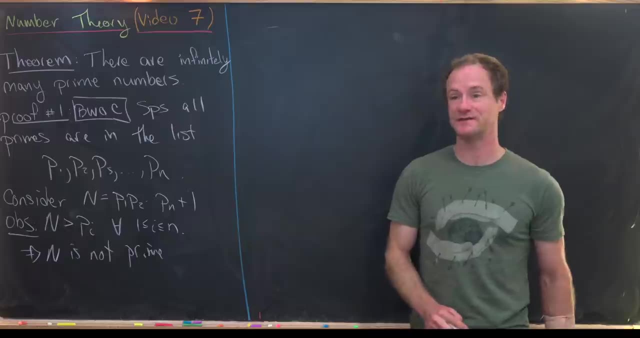 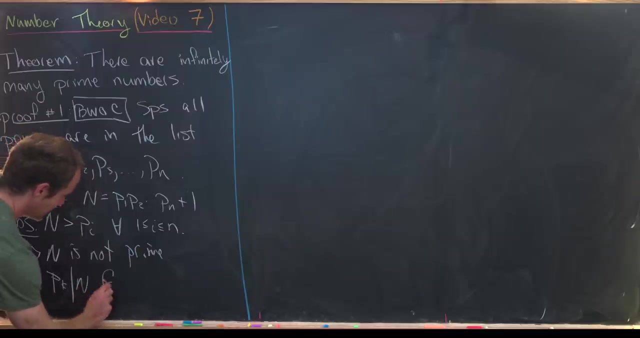 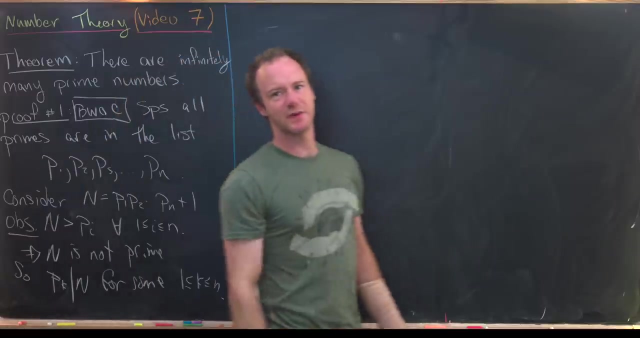 But if n is not prime- and these are all of the primes- by the fundamental theorem of arithmetic we know that one of these primes must divide n. So let's write that down. So pk divides n for some k between 1 and n. Again, that's by the fundamental theorem of arithmetic. Okay, but notice. 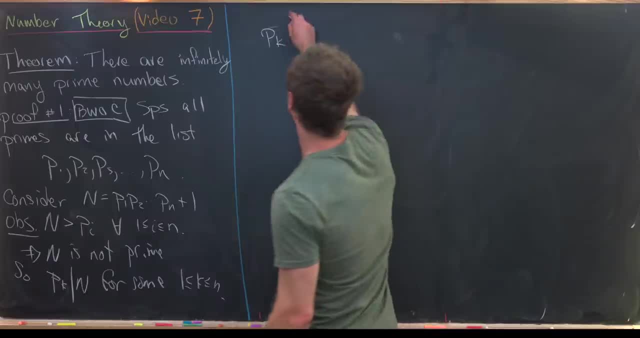 that this is not prime. So pk divides n for some k between 1 and n. So pk divides n for some k between 1 and n. Again, that tells us that pk also divides the following number by one of our results: 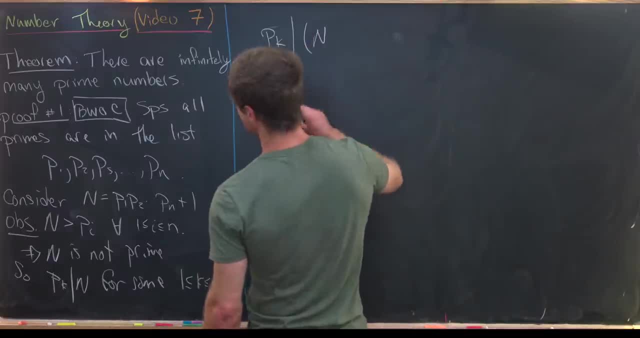 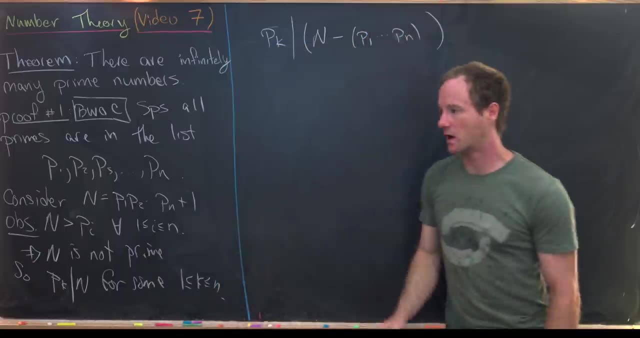 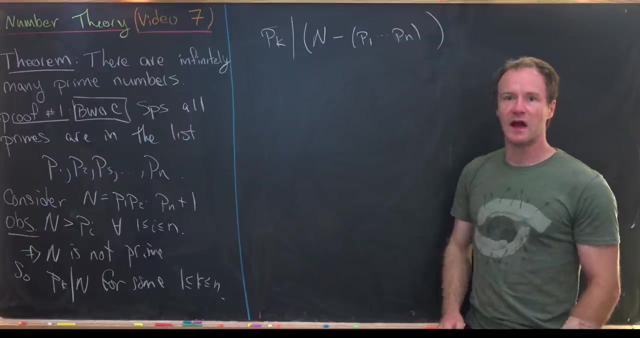 involving divisibility, And that number is going to be n minus this product, p1 up to pn. You might say: well, why does it divide this product? Because pk is one of those within that product. And then remember, if you have something that divides two numbers, it divides any linear. 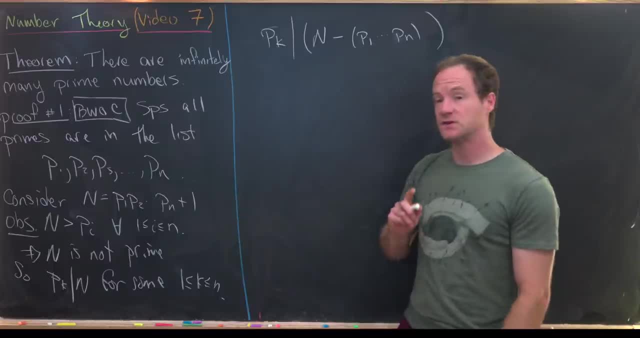 combination of those two numbers. So if you have something that divides two numbers, it divides any linear combination of those two numbers. So if you have something that divides two numbers, but that's what we've got here, So just to reiterate, pk divides n, That's like by the fact. 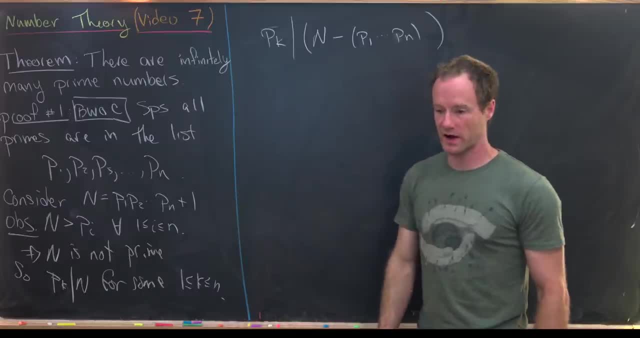 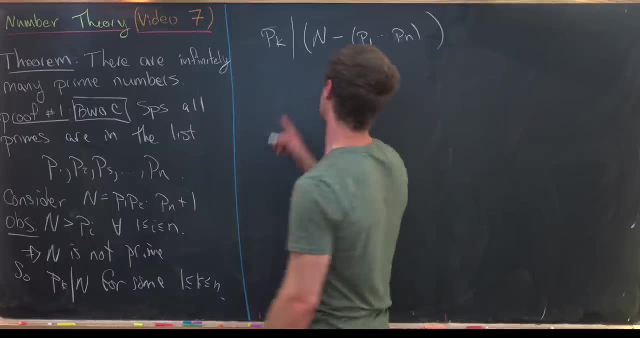 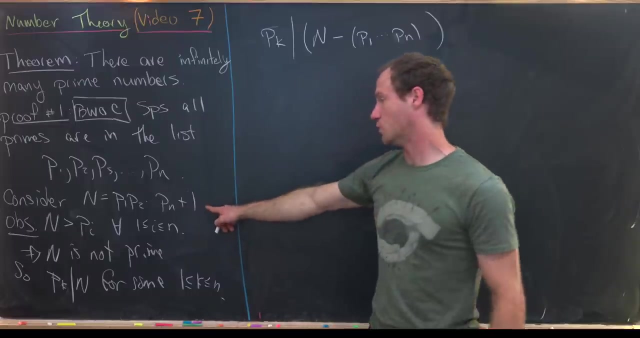 that n is not a prime. and these are all of the primes. And then pk defines this product just by the definition of divisibility. Okay, but now let's calculate this number right here. Notice that this number right here is exactly equal to 1, given the definition of capital N. So that tells: 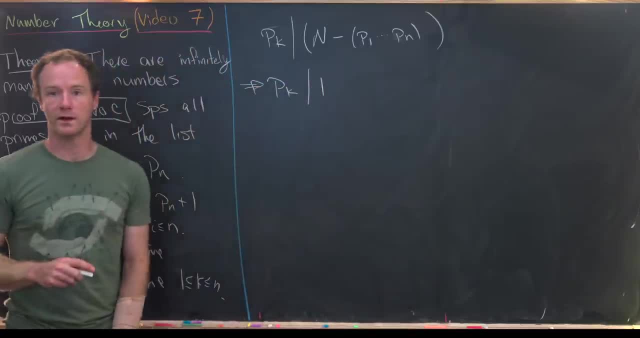 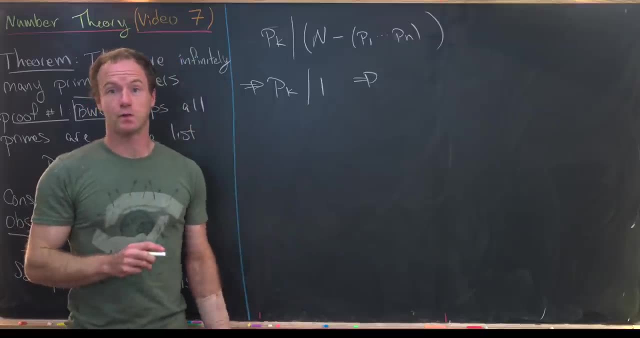 us that pk divides n, for some k between 1 and n. So that's what we've got here. And then pk divides the number 1.. But there's only one natural number that divides the number 1, and that is 1 itself. 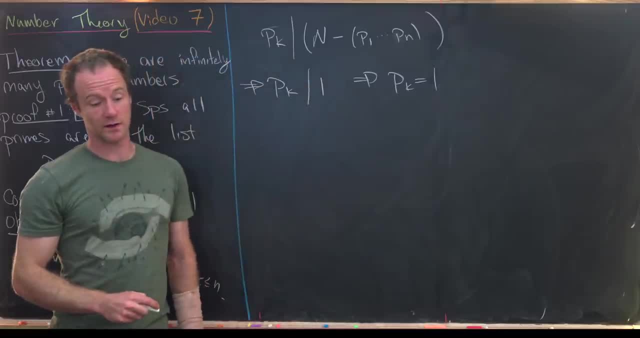 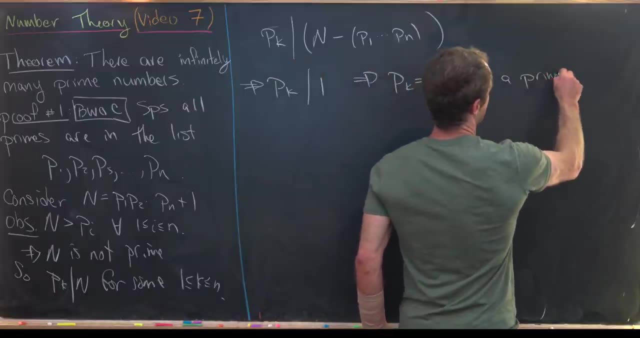 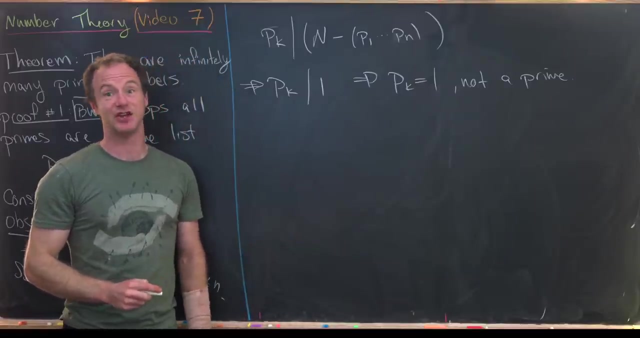 So we've got: pk is actually equal to 1.. But 1 is not a prime. Remember that natural numbers are separated into primes, composite numbers and units. Well, there's only one natural number that divides the number 1, and that is 1 itself. 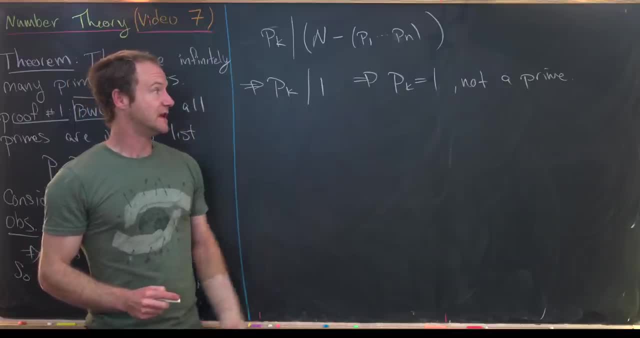 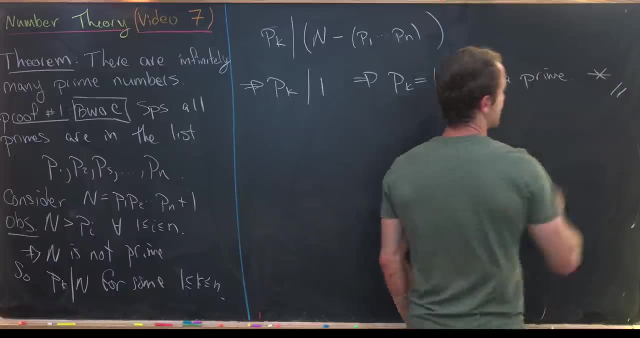 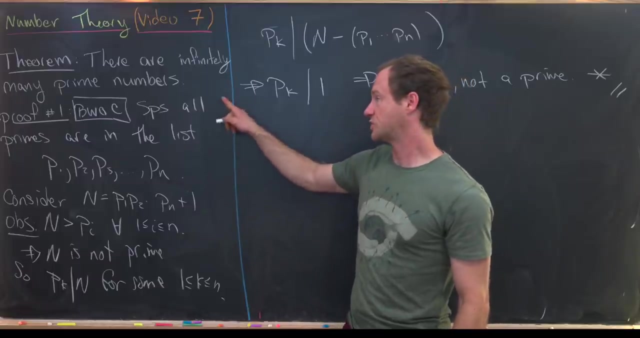 So we've got that pk is not a prime, but over here we assumed that it was a prime. So we've reached our contradiction. And you might say, well, what did we contradict? Well, we go all the way up to the start of this proof and our assumption was that all of the primes are on the 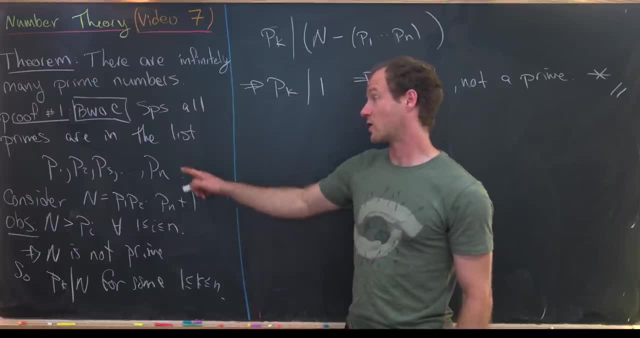 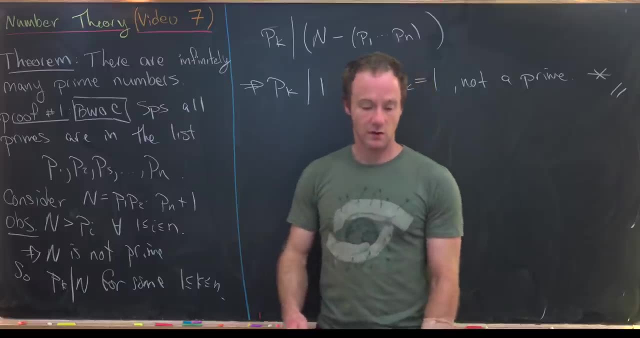 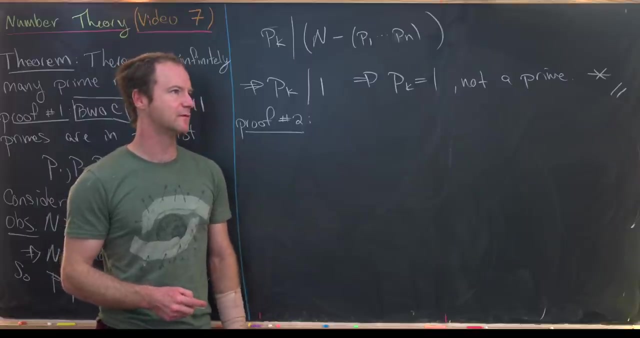 following list, But that means that there are primes that are not on this list. In other words, there must be infinitely many primes, Okay. So now that we've got this, let's go ahead and look at our second proof. Okay, Now we're going to look at a second proof. I kind of like this proof more. I don't know if 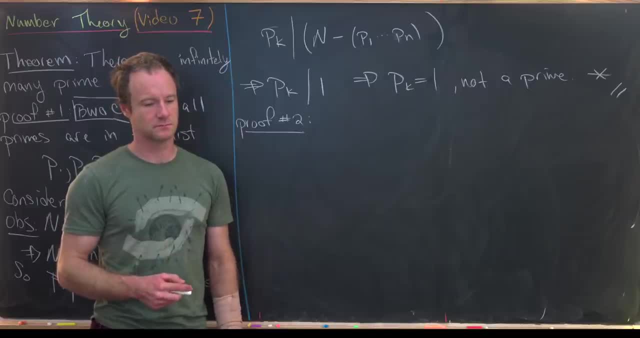 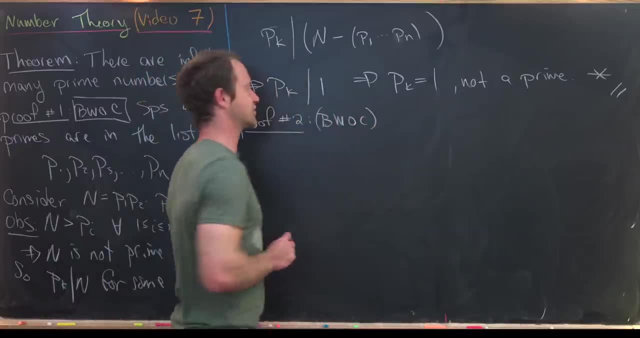 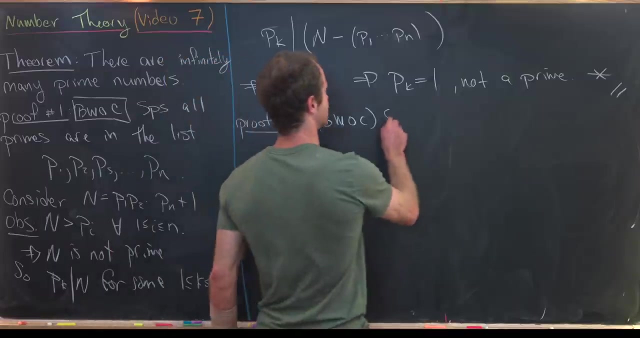 it's just because it's non-standard. Now we're ready to look at our second proof. So it will again be by way of contradiction and it will start with the same assumption that will contradict here. So in other words, we want to suppose there are. 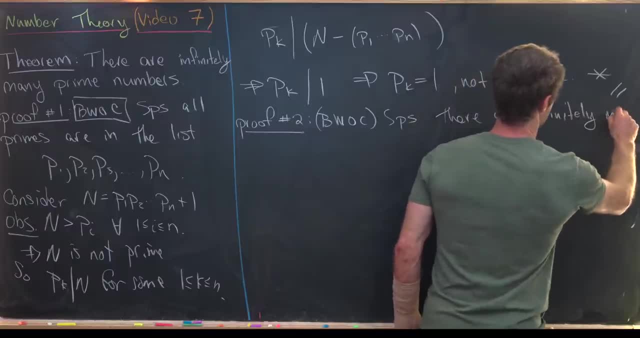 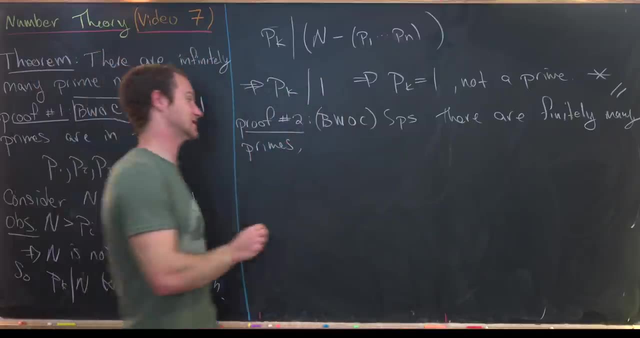 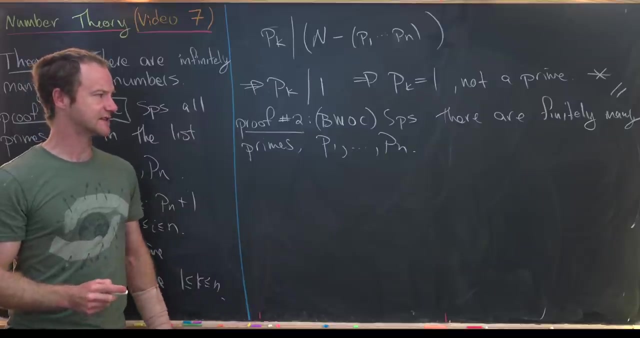 finitely many primes. And again, if there are finitely many primes, then that means that we can list them. and we'll list them the same way: p1 through pn. Now we're going to consider the following kind of interesting number, And that number I'll call it capital M, because we've 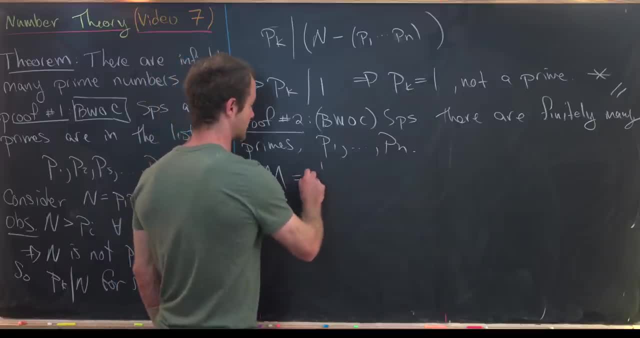 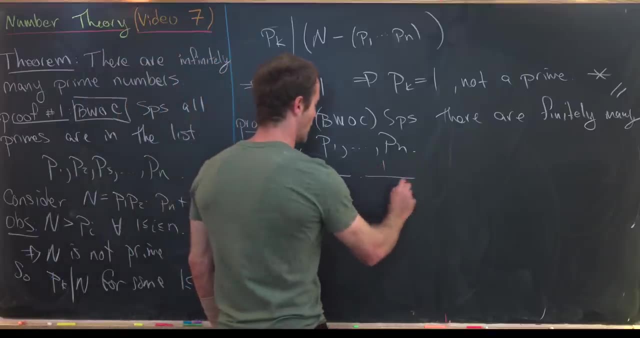 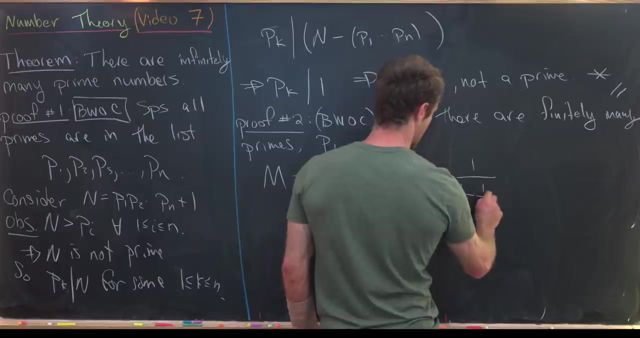 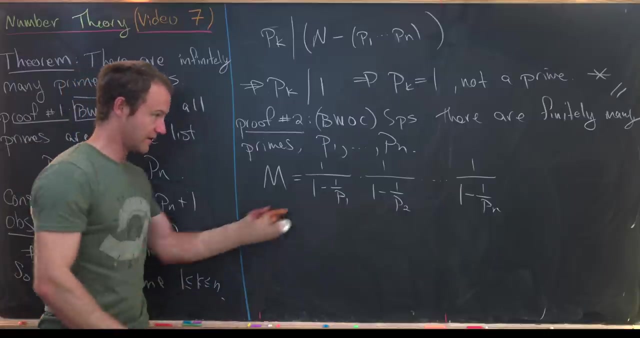 already used capital N and it'll be the following product: One over one minus one over p1, times one over one minus one over p2, times all the way up to one over one minus one over pn. So it's going to be that finite product. The important thing is that that is a finite. 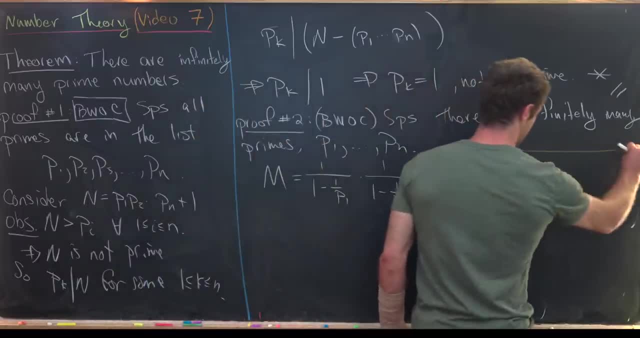 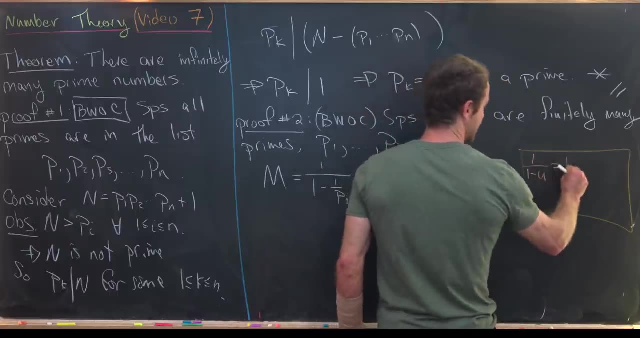 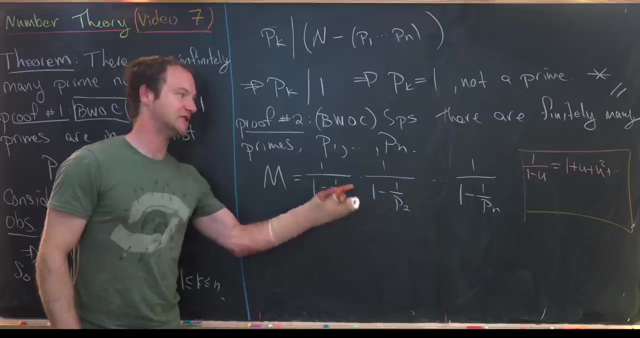 product. But now we can use the standard formula for the sum of the geometric series to write one over one minus u, And that's going to be the sum of the geometric series, And that's going to be as one plus u plus u squared, and so on and so forth, And apply that to each of these parts of 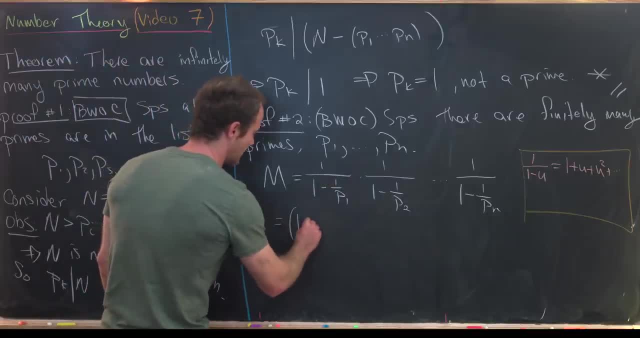 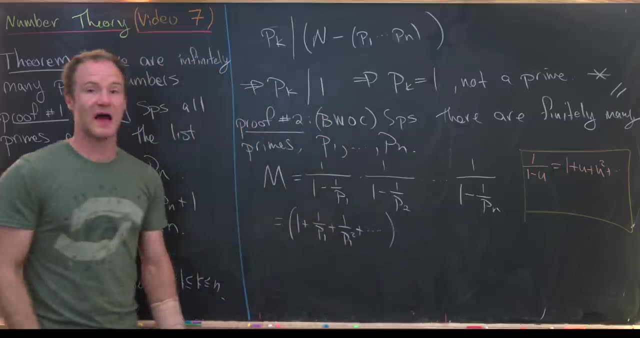 the product. So we've got- this is one minus, or sorry, one plus one over p1, plus one over p1 squared, plus dot, dot, dot, all powers of one over p1.. And similarly, here we'll have all powers of. 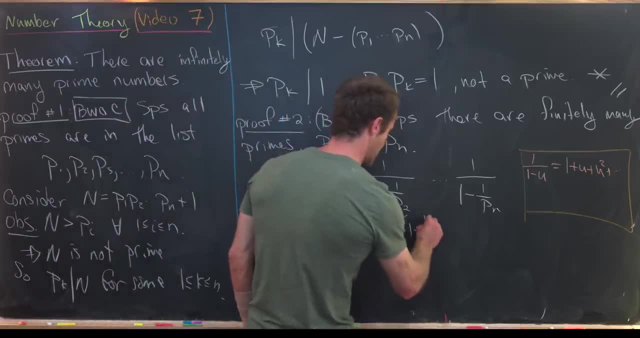 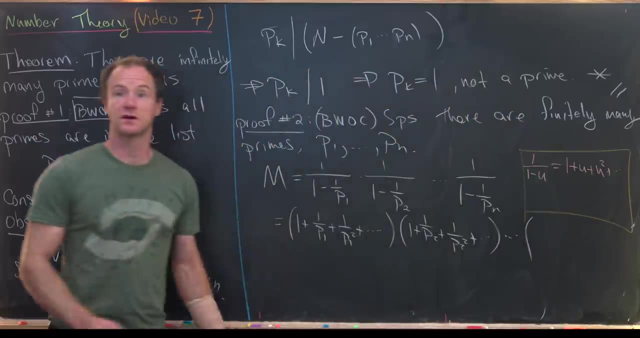 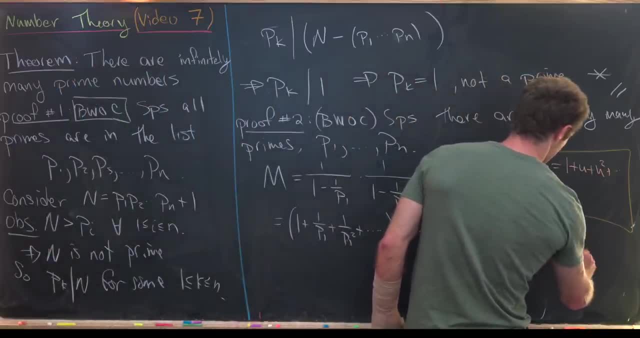 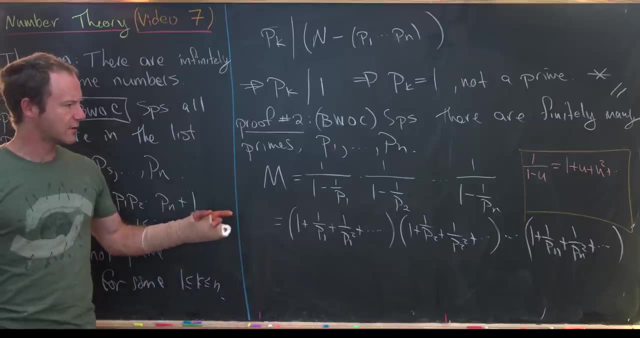 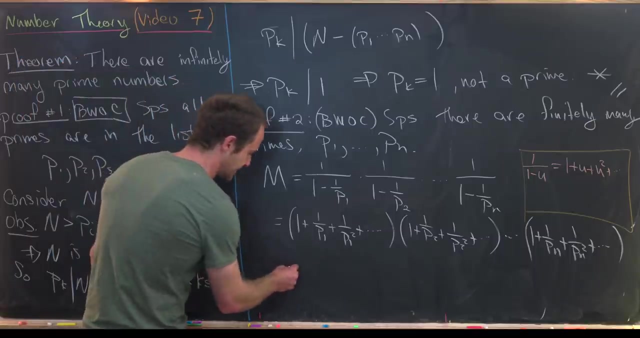 got one plus one over pn, plus one over pn, squared plus all the way up, Okay. But now notice, if we were to just expand this entire product, we would get exactly the harmonic series. So this is going to be equal to one plus one half. 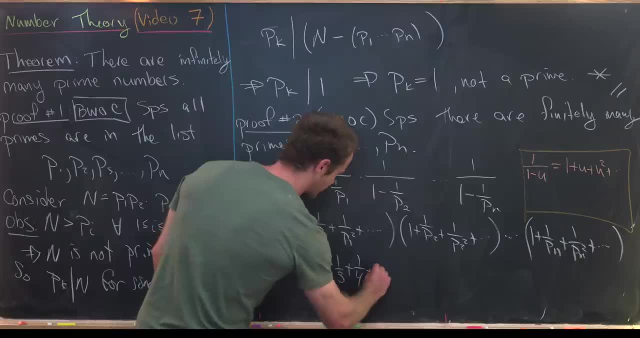 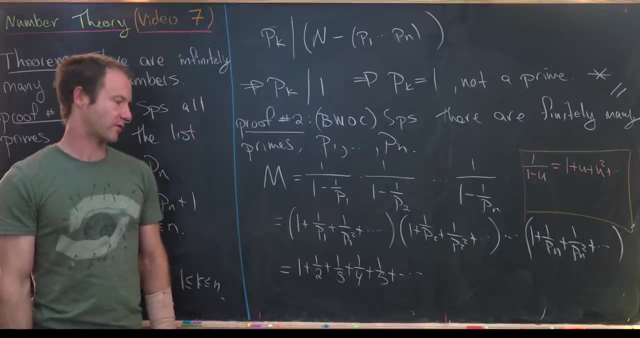 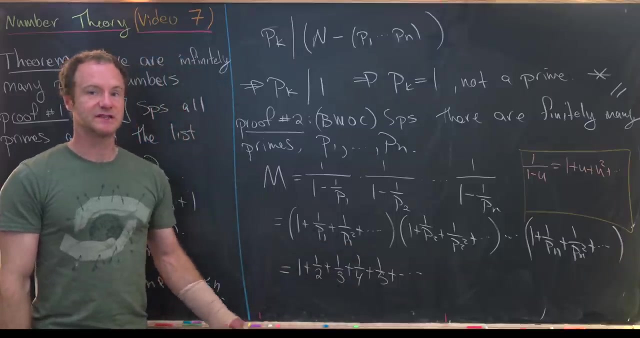 Plus one third, plus one quarter, plus one fifth, and so on and so forth. So how do we know that? Well, that's by the fundamental theorem of arithmetic. So we could pick a natural number, and the reciprocal of that natural number is only created by one term from this huge product. 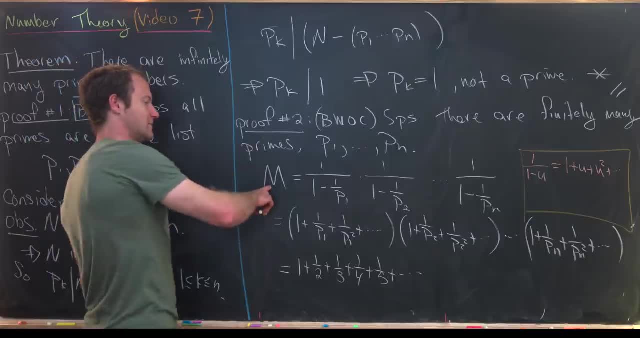 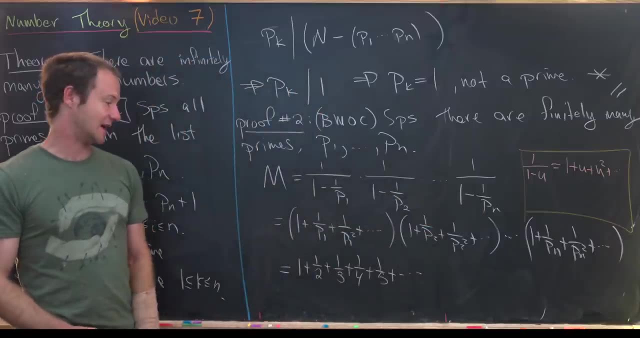 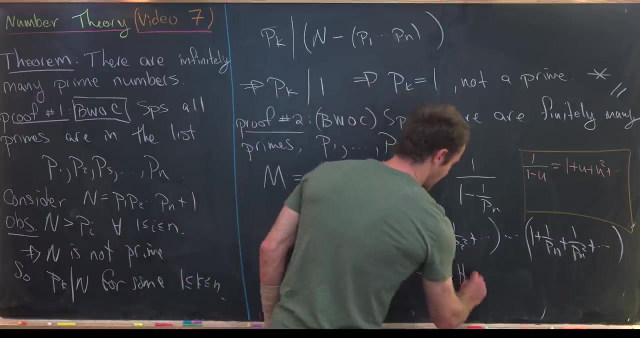 Okay, But let's see what we've got here. We've got this number: m is a finite product of positive numbers. That means it's a finite number, but it's also equal to the harmonic series. So what did we just do? We just proved that the harmonic series converges. 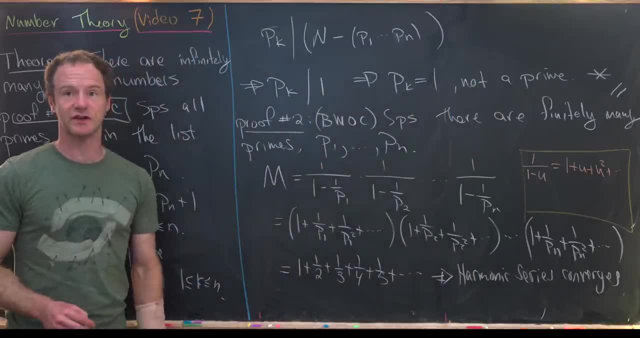 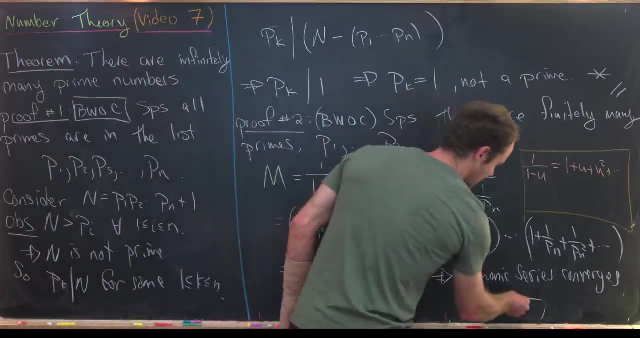 But that's a problem, because any calculus two student, well, at the end of calculus two, knows that the harmonic series does not converge. So that means we've reached a contradiction. And what did we contradict? Well, going up to the beginning of the proof, we contradicted this. 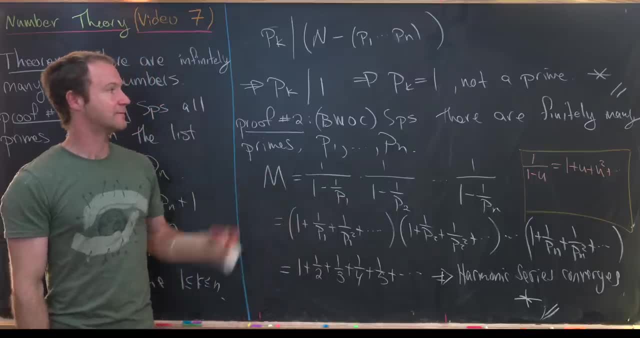 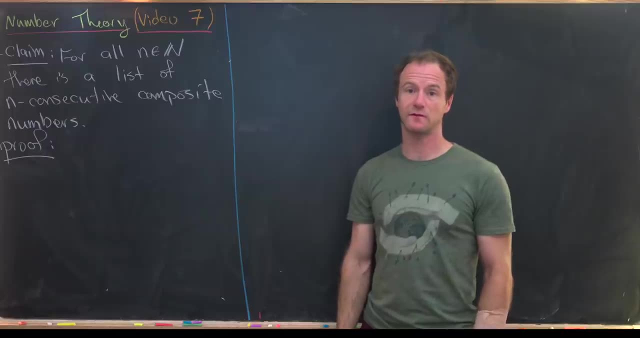 assumption that there are finitely many primes. Okay. So now that we've got this taken care of, we're going to look at a couple more results. So one thing that we noticed in our last proof, or our last proofs, was that those proofs were not constructive. So what I mean is that we 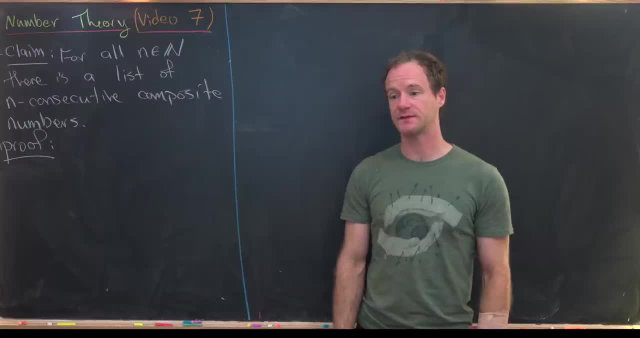 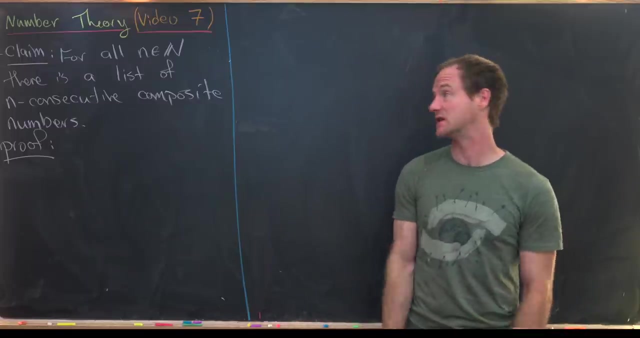 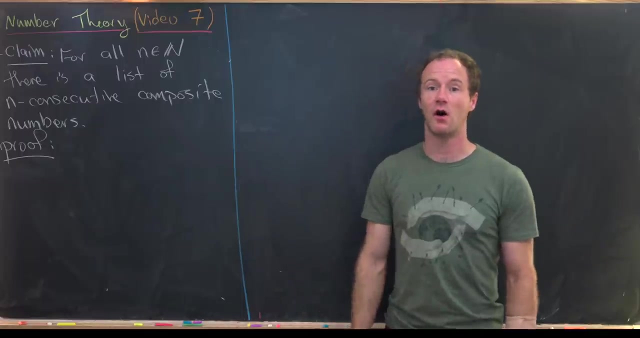 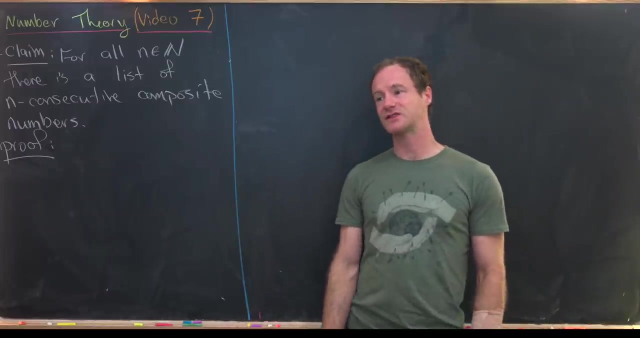 proved indirectly that there are infinitely many primes. And we did it that way because there's no real constructive proof. So we're going to look at a couple more results. So let's look at a couple more results. So what do I mean by that? Well, let's notice that if we take eight, nine and ten, 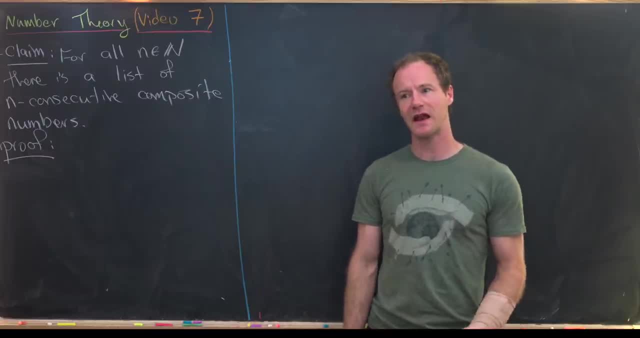 those are three composite numbers. So what do I mean by that? Well, let's notice that if we take eight, nine and ten, those are three composite numbers in a row. And you might ask yourself the question: is there some sort of upper limit for how many composite numbers that you can have in? 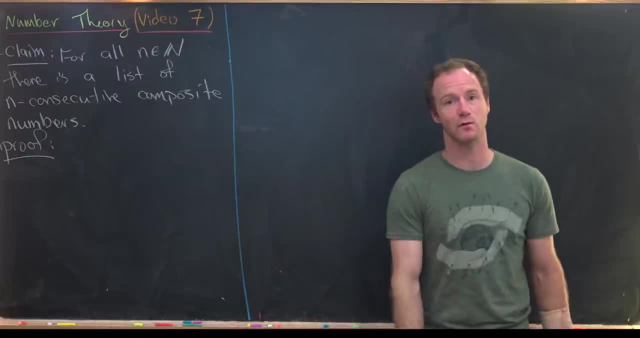 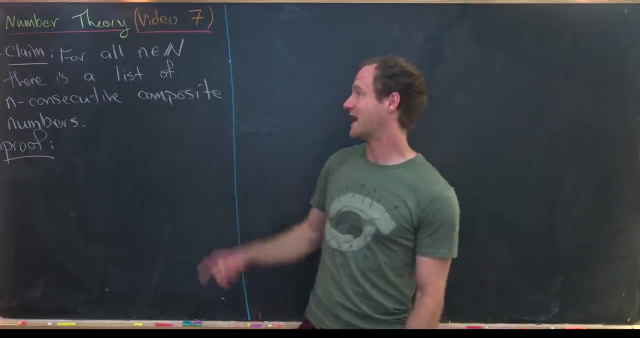 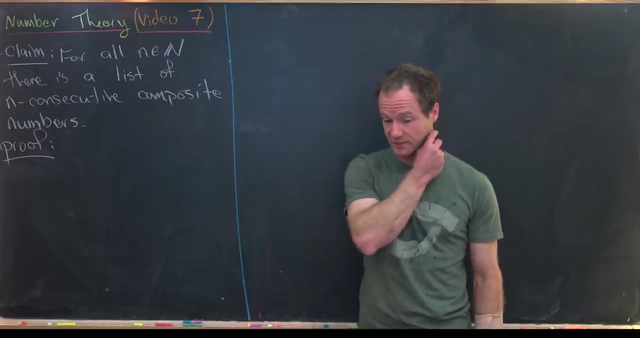 a row, And in fact there isn't, And that's what this claim will prove. So let's look at the careful statement here. So, for all natural numbers n, there is a list of n consecutive composite numbers And, as I alluded to, this is going to be a constructive proof. So what we'll? 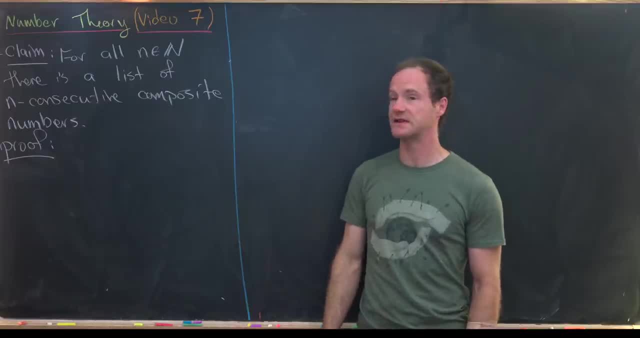 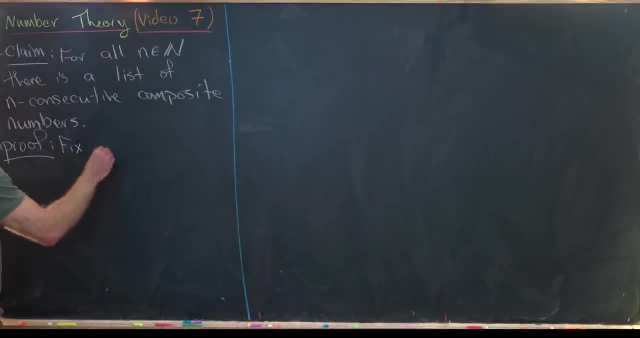 do is we'll just construct a list of n consecutive composite numbers And, as I alluded to, this is going to be a constructive proof. So let's do it. So let's maybe fix our n, which is a natural number, And now we can just like make a list of n consecutive composite numbers, And we can do it. 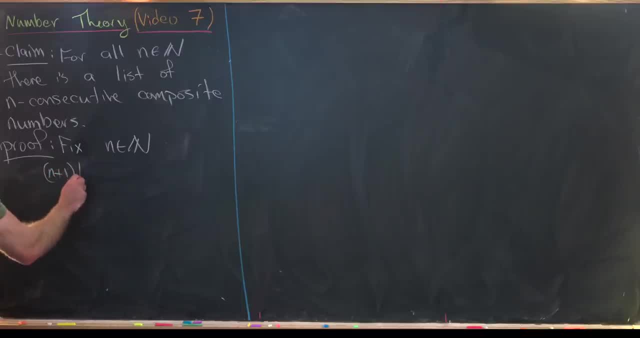 in the following way. We'll take n plus one factorial plus two. Well, let's notice that n plus one factorial will definitely be a multiple of two, because n plus one factorial is a multiple of two. So that means we can write this as two times something. I'll just write it like that, And 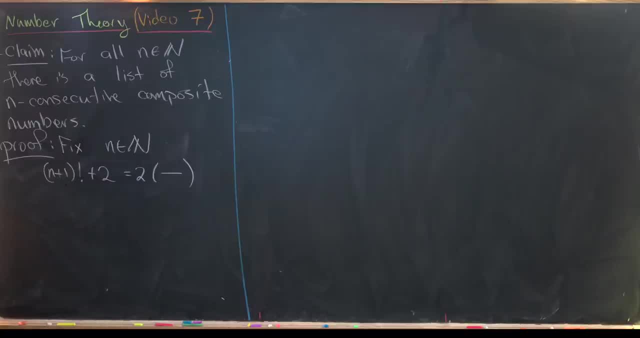 that's because this is divisible by two and this is divisible by two, And now we can just keep playing that game. We'll take n plus one factorial plus three, And then, if n is large enough, n plus one factorial is divisible by three. So that means we can factor a three And then we can. 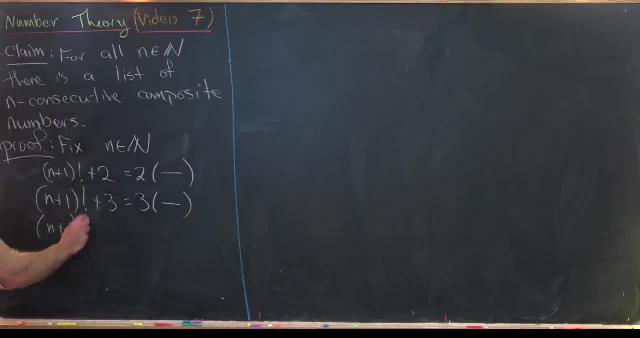 three out, And then likewise n plus one. factorial plus four can have a four factored out of it, as long as n plus one is long enough. Obviously, this list is not going to last forever, So we really want to think about how long it will last. And it will last up until we're adding n plus one. So 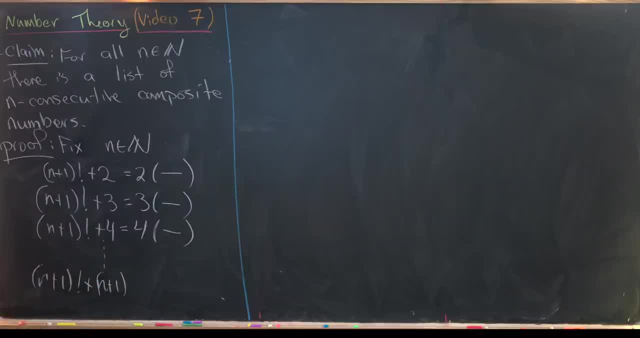 notice: n plus one factorial is definitely a multiple of n plus one, And so we're going to have n plus one factorial plus three. So that means we can factor an n plus one out of this, And then we have something left over. But now let's count up how many we have on this list. Well, we 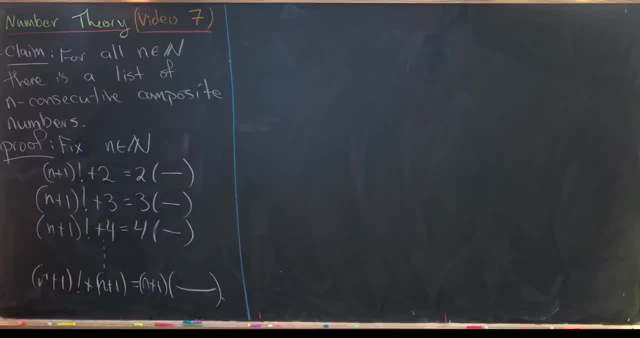 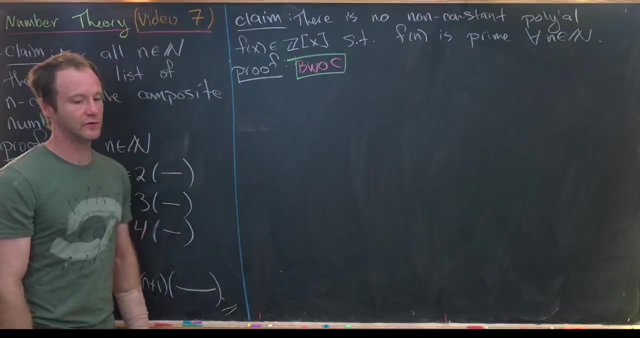 start at two, We end at n plus one. So that means we've got a total of n elements in this list And we've written all of them in a factored form, meaning that they are all composite. Our next little claim that we'll prove will give evidence towards the fact that n plus one factorial is. 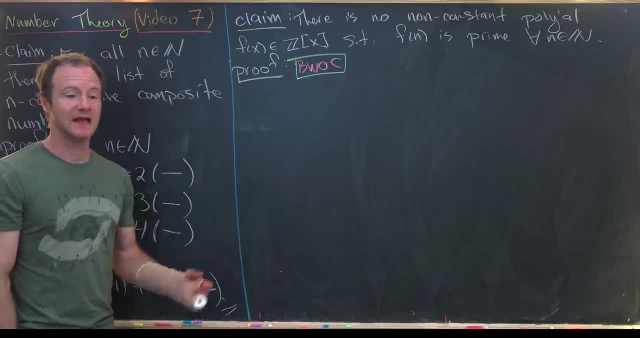 not constant. We're going to stick with the fact that it is constant, so that we can also draw up the ticket point. So what we want to do in this table? we want to say that there's no polynomial that will always generate prime numbers. That's fine. We've already got a. 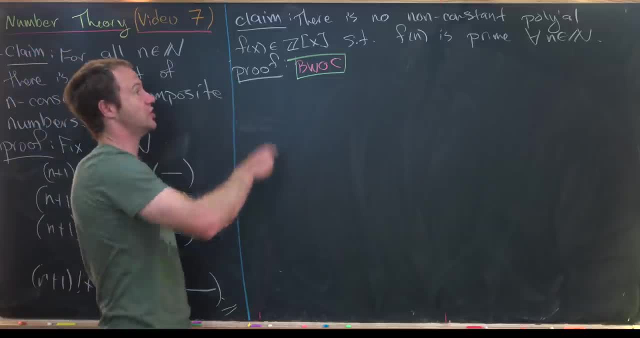 polynomial that we want to draw up. So we want to say that there is no polynomial that will always generate prime numbers And in fact, what we'll do is show that there is no polynomial that will always generate prime numbers. So, more carefully, we could say that like this: There is no. 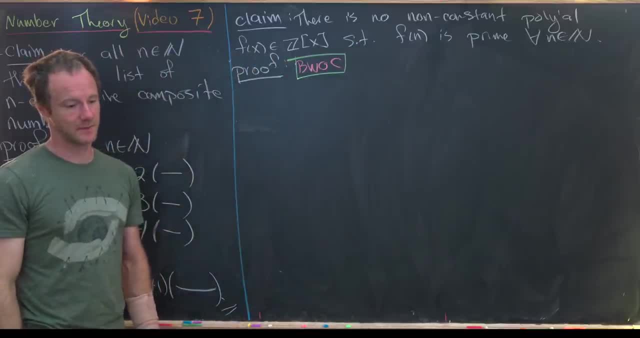 non-constant polynomial f of x in z adjoining x. So what I mean by that is, f has coefficients that are all natural numbers in. Okay. so let's maybe see how we can do this Again. we're going to do this. 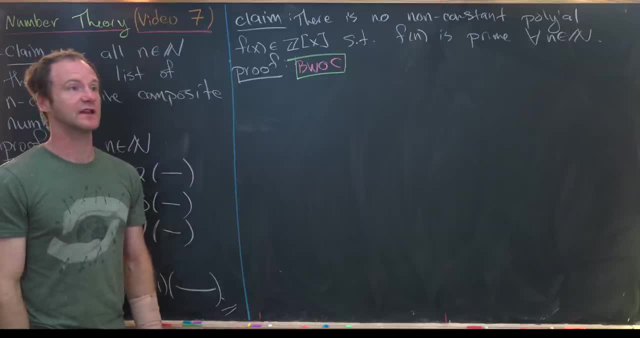 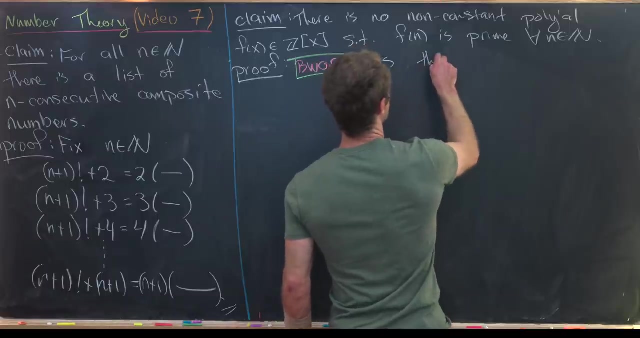 by way of contradiction. So this is like a really So proving things by way of contradiction is a really powerful tool, as we'll see moving through this course. Okay, so let's start off by supposing that there is some f of x in z adjoining x, in other words, a polynomial with 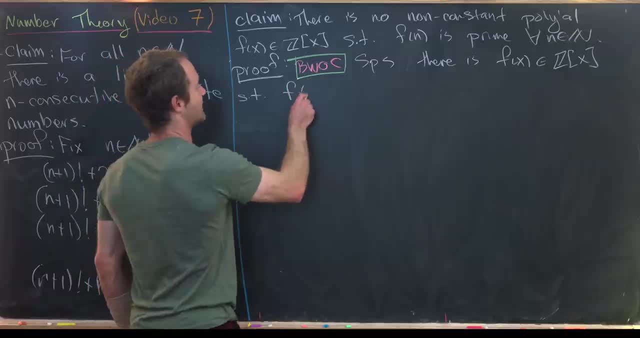 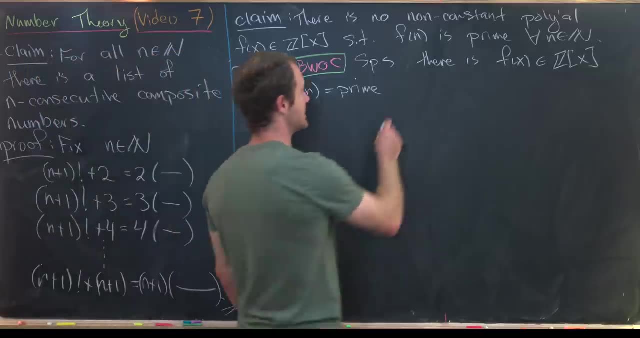 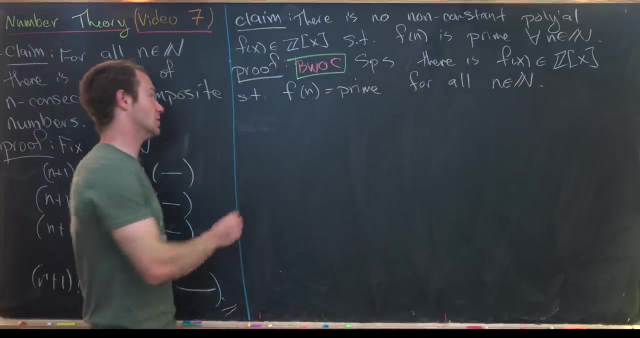 integer coefficients such that f evaluated at n is equal to some prime. I'll just say: f of n equals a prime for all natural numbers in. Okay, so what does that mean? Well, the number one is a prime, so that means that f of n is equal to a prime for all natural numbers in. 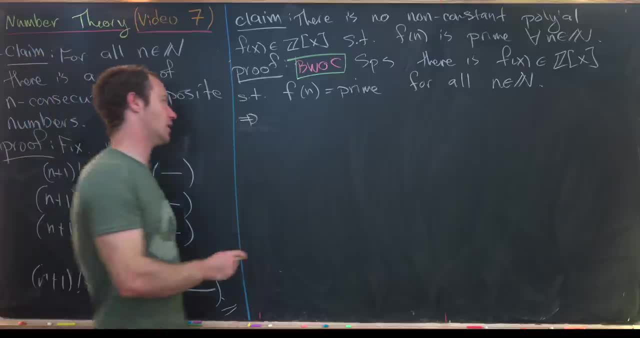 Well, the number one is a prime. so that means that f of n is equal to a prime for all natural numbers in a natural number. So that means f evaluated at 1 is a prime. So I'll just say f of 1 equals p. 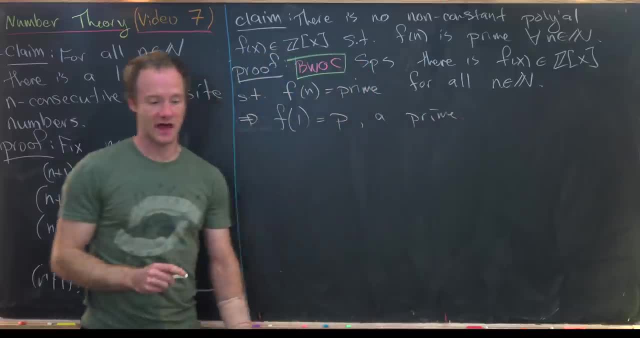 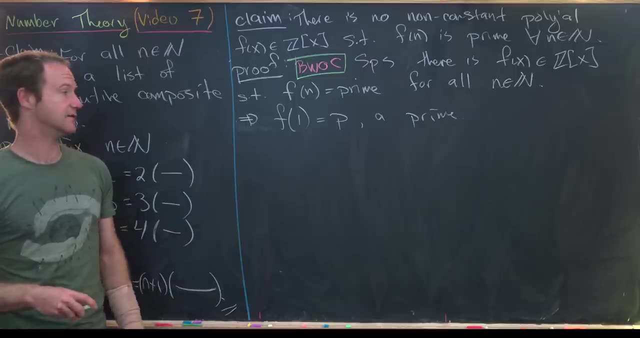 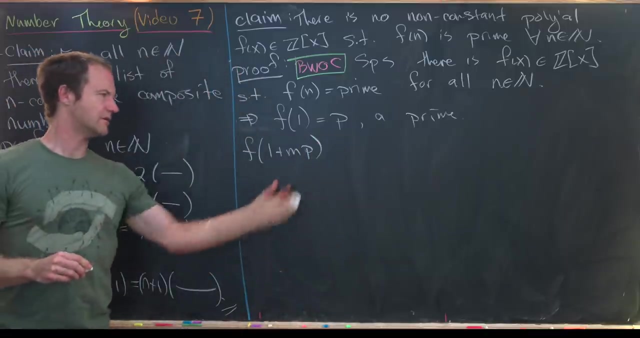 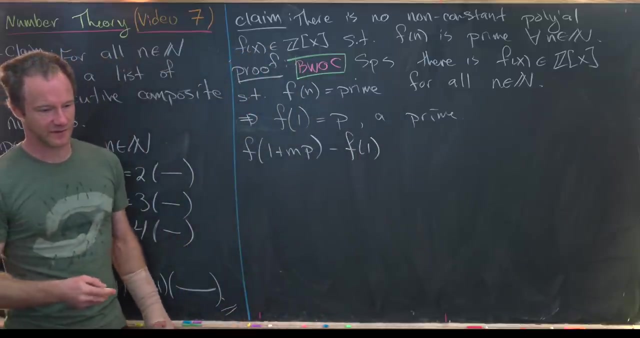 a prime number. So we'll give a name to f evaluated at 1.. And now, next, we want to look at the following: difference of values of f. So we'll look at f of 1 plus m times p- sort of m times p, for obvious reasons- minus f evaluated at 1.. So let's see what we get for this. 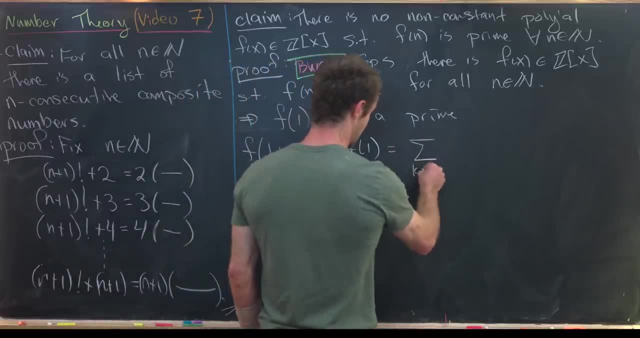 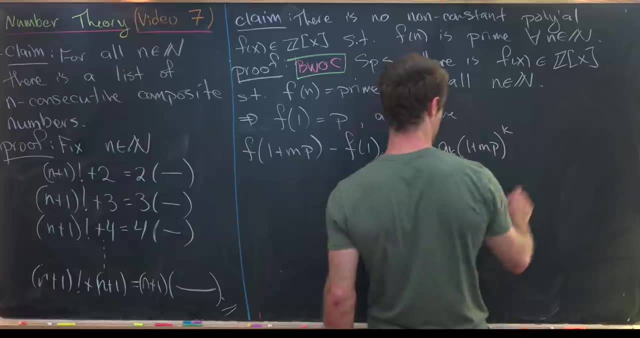 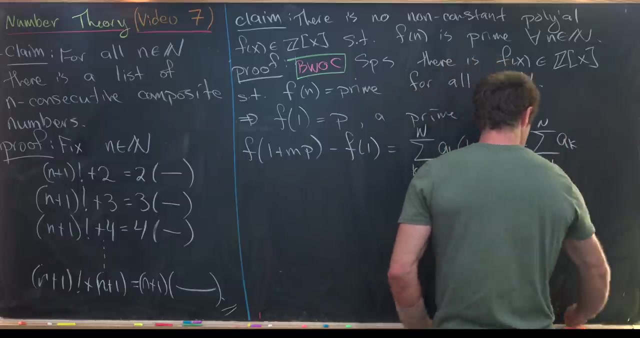 So that's going to give us this sum as k goes from 1 up to n of a k, 1 plus m p to the k minus this sum as k goes from 1 up to n of a k. And so here I've kind of built into this notation. 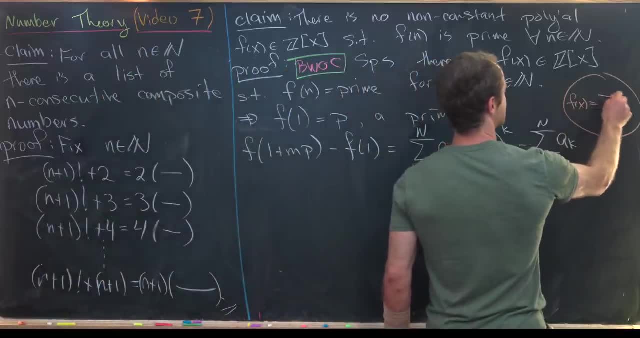 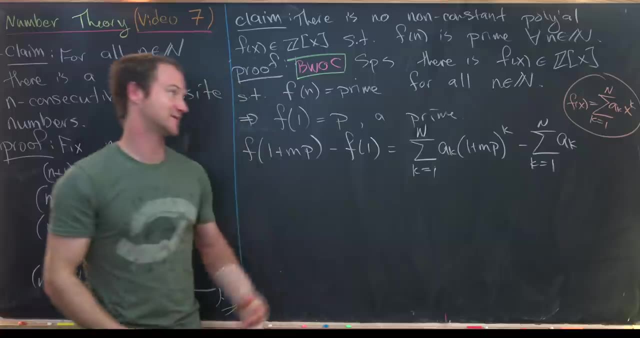 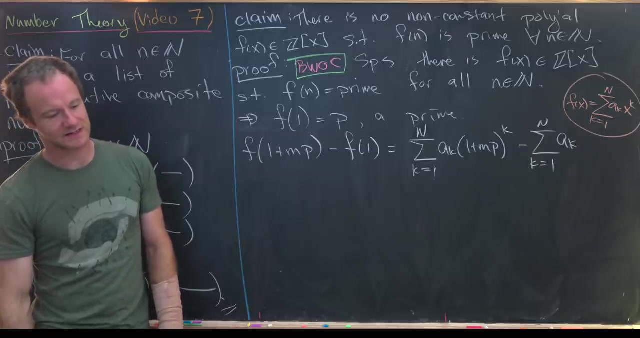 that f of x is equal to this sum, as k goes from 1 up to n of a k, x to the k. So that's just like a standard way of writing a polynomial down in summation notation. Now let's see if we can simplify that. So I'll start by combining those two sums together. 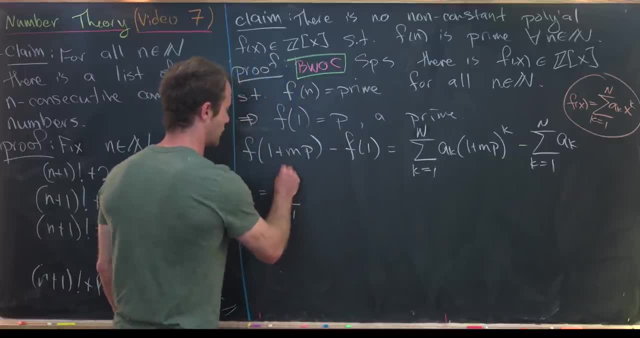 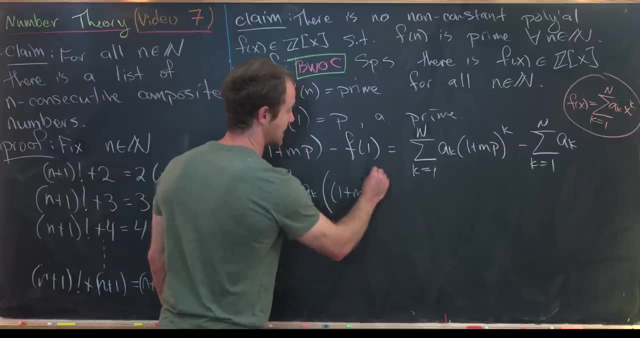 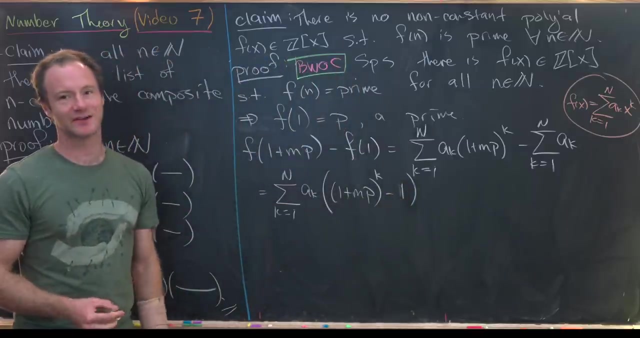 That's going to give me this sum, as k goes from 1 up to n, of a k times the quantity 1 plus m p to the k minus 1.. So again, I just push those two sums together and then factor the a k. 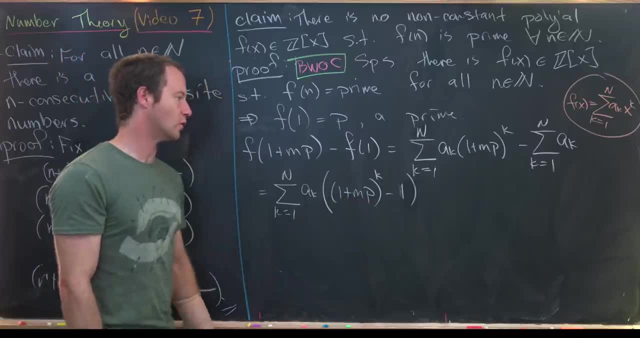 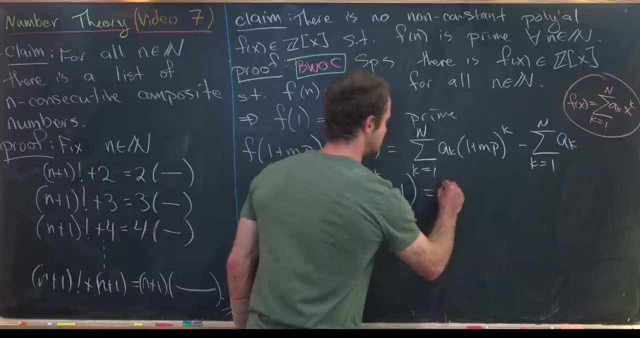 out. But now I can take this binomial 1 plus m p to the k and expand it using binomial coefficients, And so I'll have a sum within a sum. So just to write that more carefully, I've got this sum as k goes from 1 up to n of a k And then 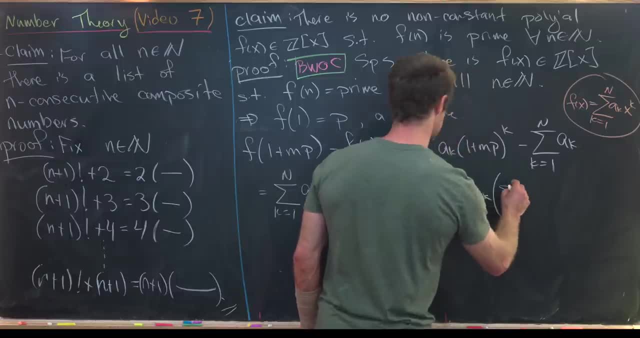 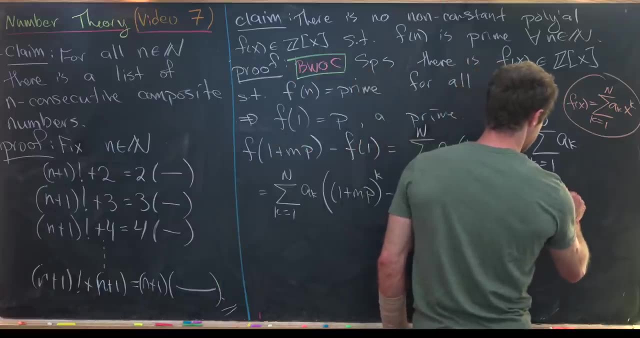 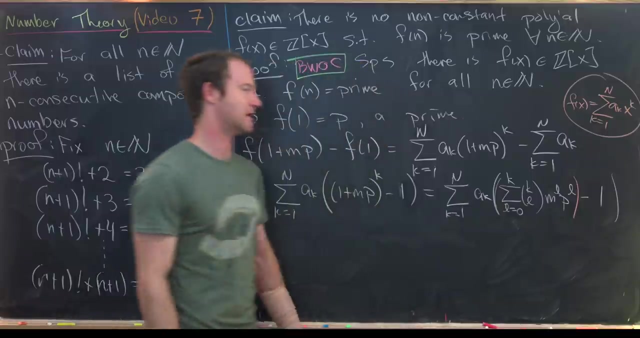 inside of that I'll have this sum as l goes from 0 up to k of k, choose l m to the l, p to the l minus 1.. And I'll put this sum in parentheses just to show that my minus 1 is happening outside of. 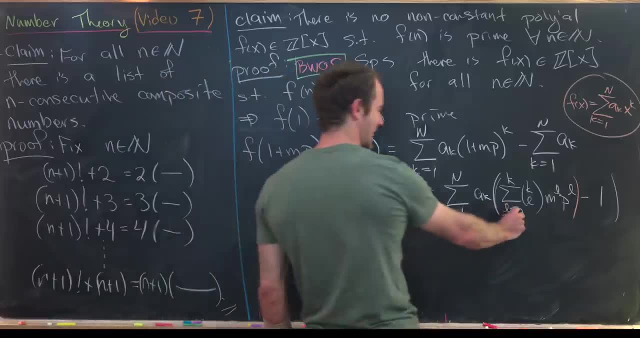 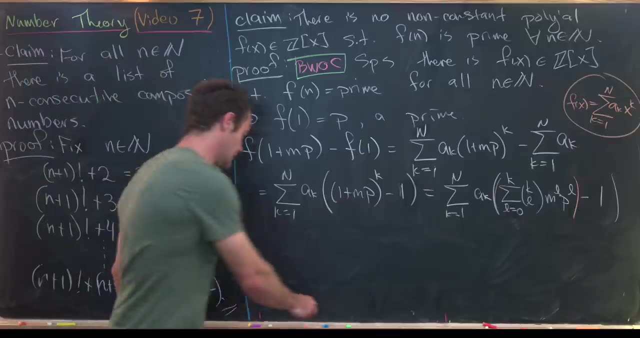 that sum. Next, I want to notice that at the l equals 0 spot I've got k choose 0, which is 1, m to the 0, p to the 0, which is also 1.. So that's going to cancel out the 1 that's out here. So that'll cancel this starting point from. 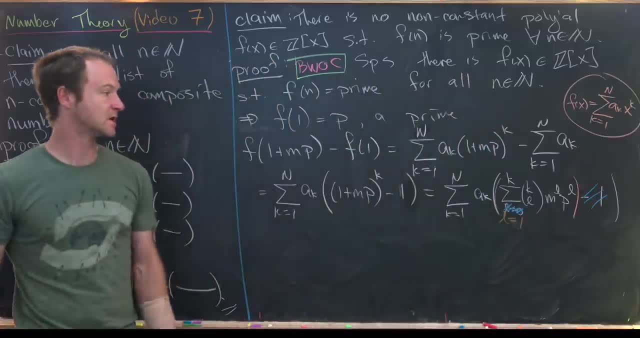 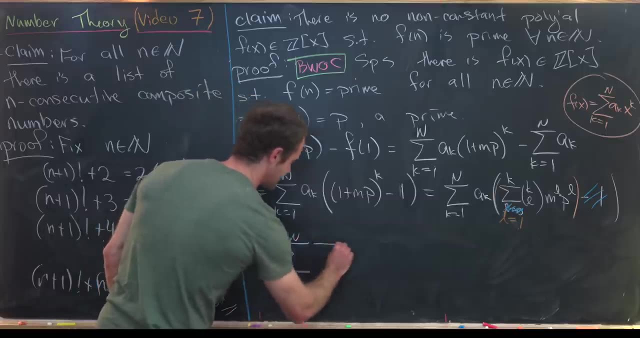 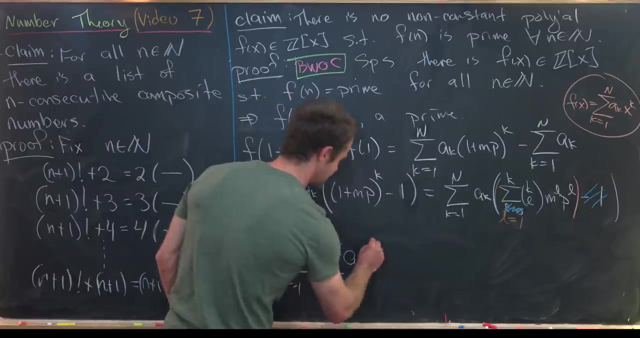 l equals 0 to l equals 1.. So that means I can rewrite this as the sum as k goes from 1 up to n, And then inside of that we have the sum as l goes from 1 up to k of a k, and then k choose l. 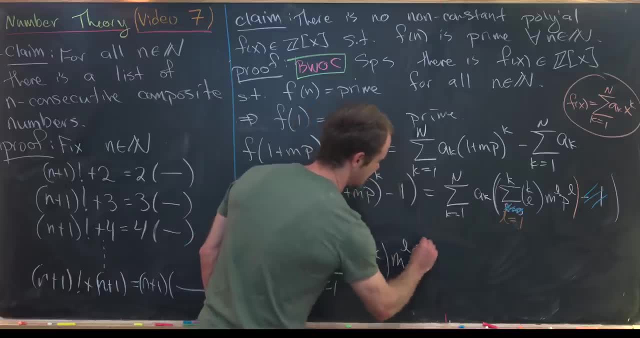 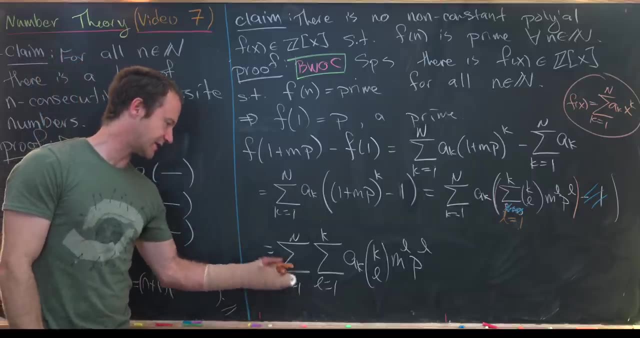 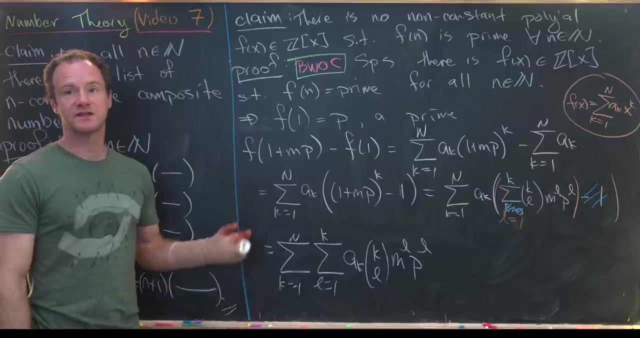 that's a binomial coefficient: m to the l, p to the k. Now, a little tricky thing that happened here is that we never had to consider the k equals 0 term. That's because that canceled out at this stage right here. Notice: the k equals 0 term is the. 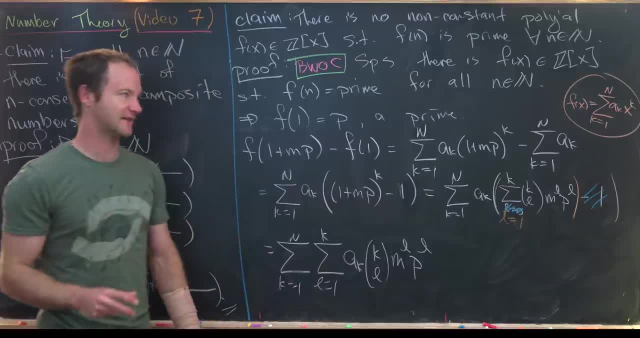 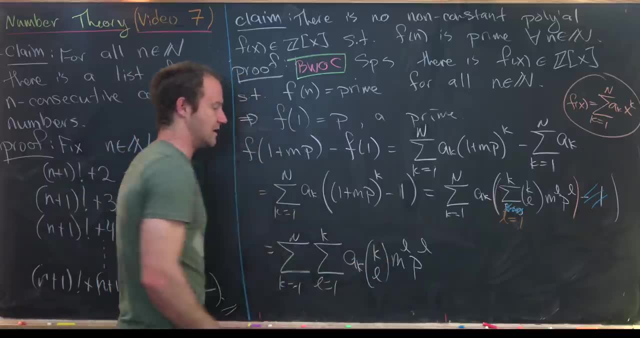 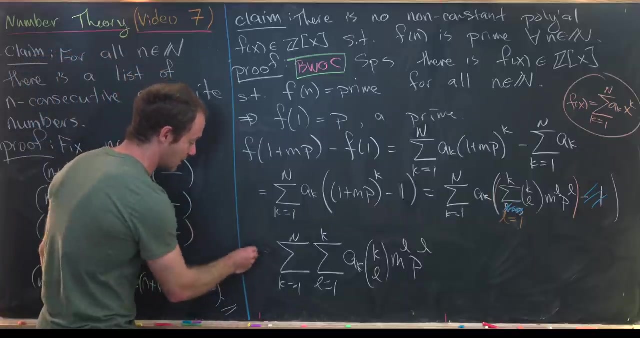 constant term of the polynomial, But whenever you take a difference like that, that constant term will cancel. So what does that mean? That means that every term in the sum has at least one power of the prime p. But that means we can factor out a p from every term in the sum And that leaves us with p to the 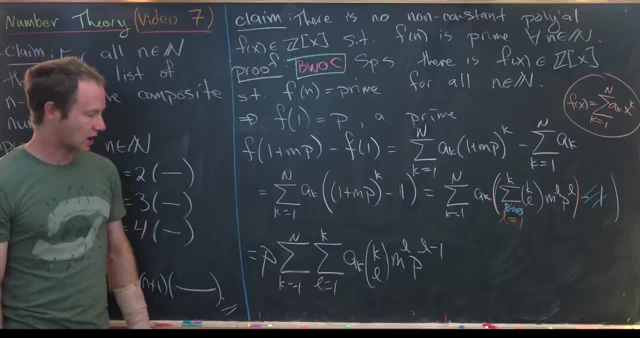 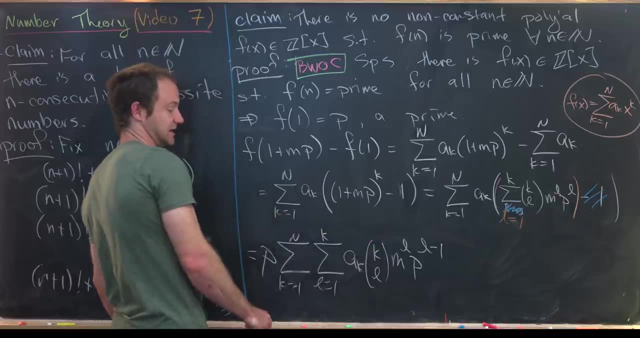 l minus 1 on the inside. So let's just talk our way through it. a sub k is an integer, k choose l is an integer, m to the l is an integer, And then p to the l minus 1 is also an integer. Again. 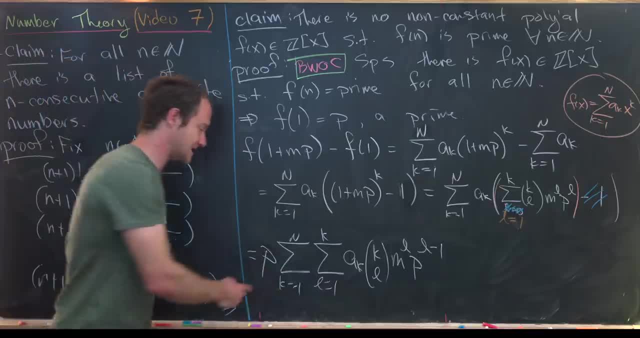 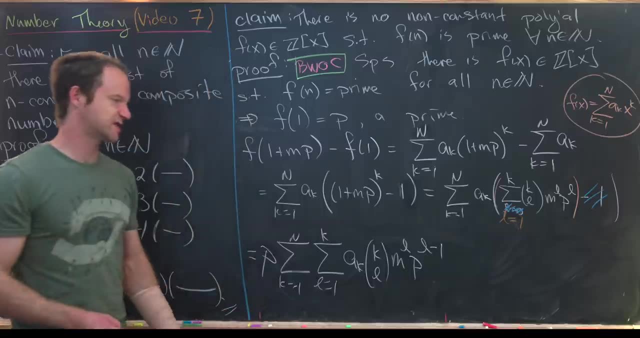 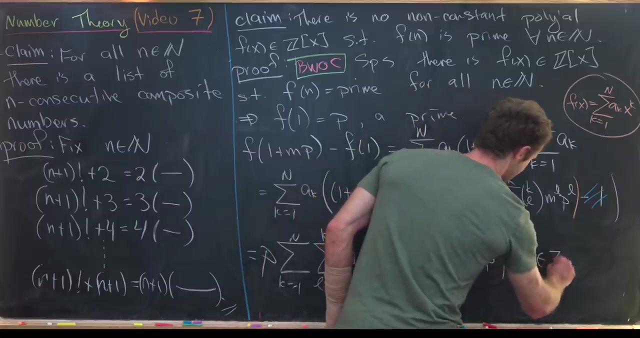 that's because l starts at 1.. But that means that this whole thing right here is an integer, So maybe we'll replace it with capital M, just to notate that that's an integer in the end. So we have: this is equal to capital M, times p, where capital M is an. 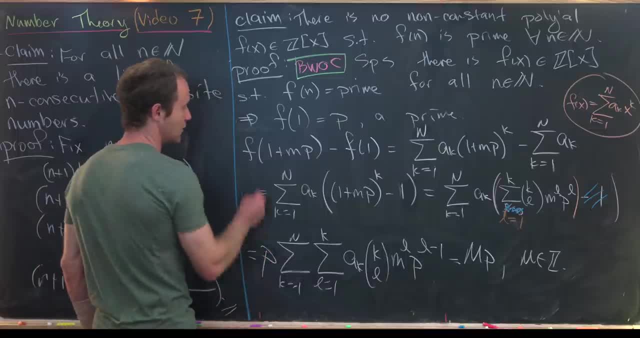 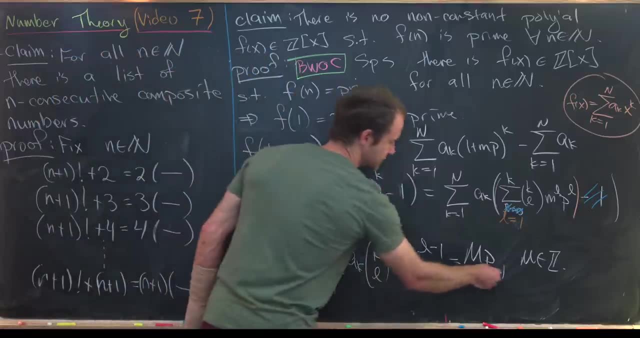 integer. So let's see what we've got so far. We have f evaluated at 1 plus m p. minus f evaluated at 1 is equal to this capital M p. But let's recall that this f evaluated at 1 is an integer. 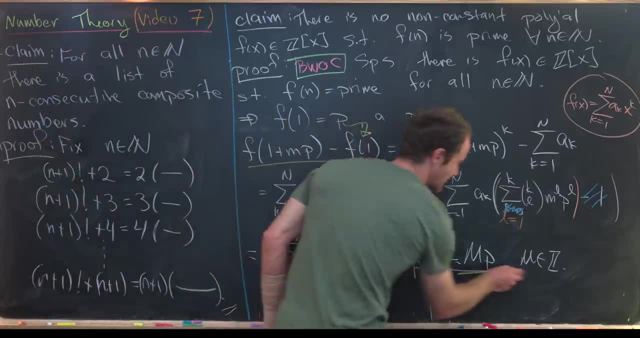 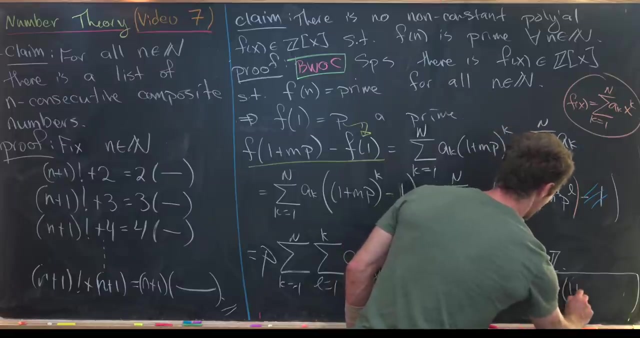 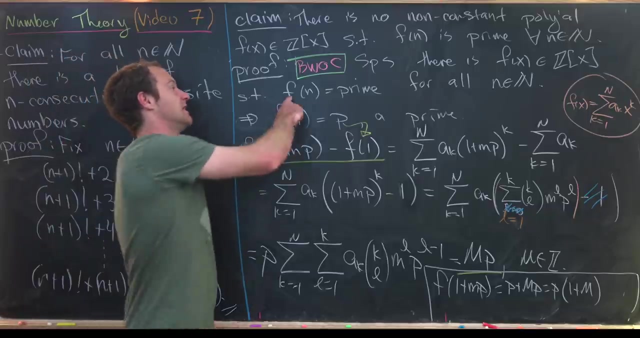 So we can rewrite this equation as follows. We can write f of 1 plus little m- p is equal to p plus capital M, p which is equal to p, and then 1 plus capital M, just factoring the p out. But let's recall that f, evaluated at n, is supposed to be prime for all natural numbers. 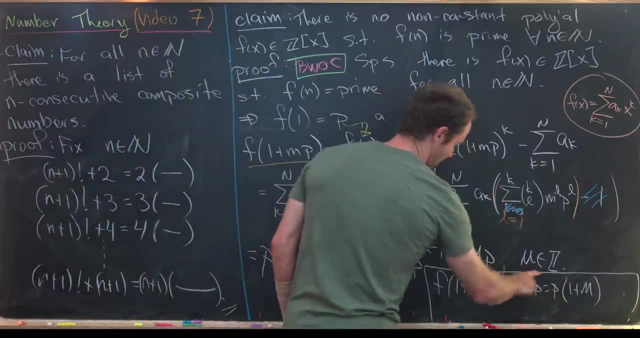 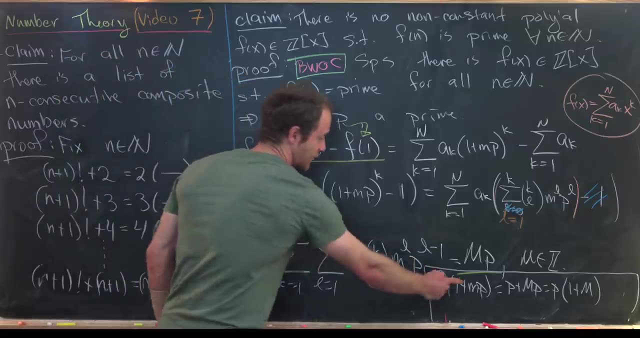 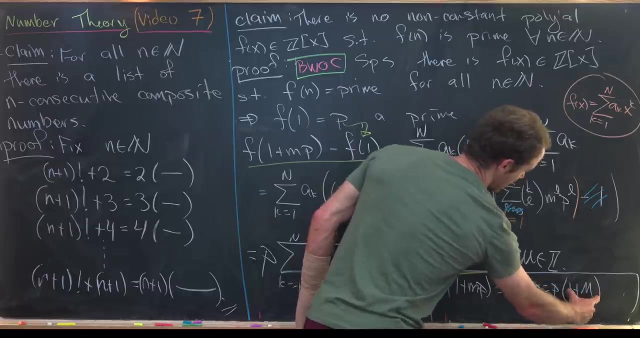 n. But what we have is that this prime divides f evaluated at 1 plus m p. But now f evaluated at 1 plus m p is most definitely not a prime, unless m is equal to 0. And this cancels down just to 1.. 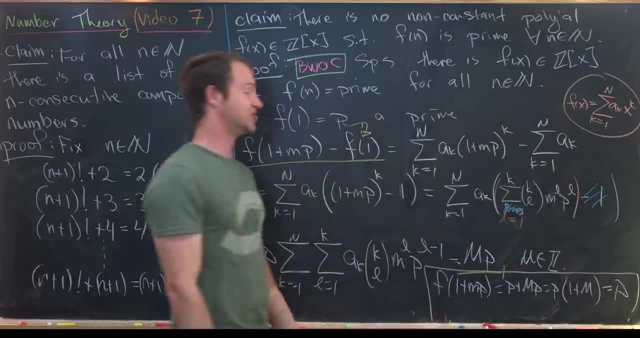 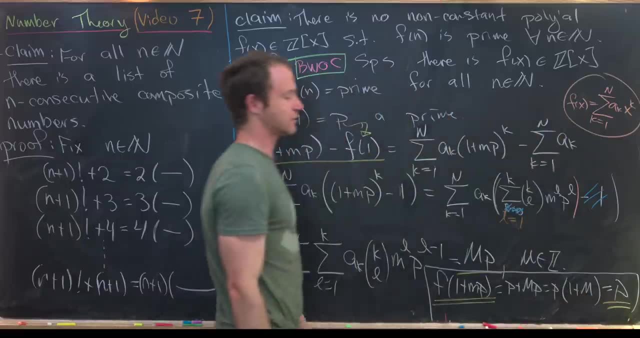 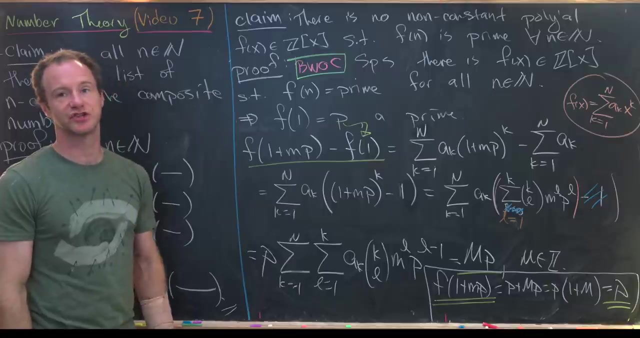 And in that case this is equal to just the prime p. So that means we've got infinitely many values of our polynomial. If our polynomial is equal to our kind of starting prime p, but if infinitely many values of our polynomial is equal to the starting prime, then that means that our polynomial was constant from. 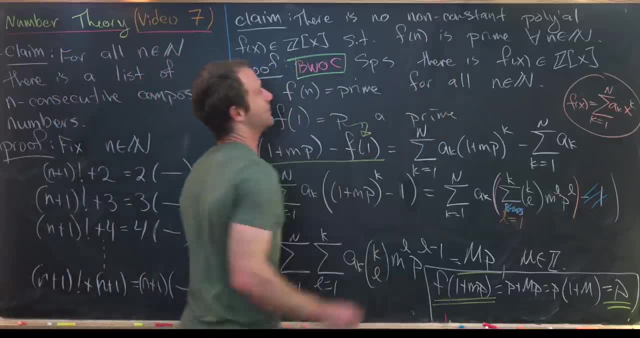 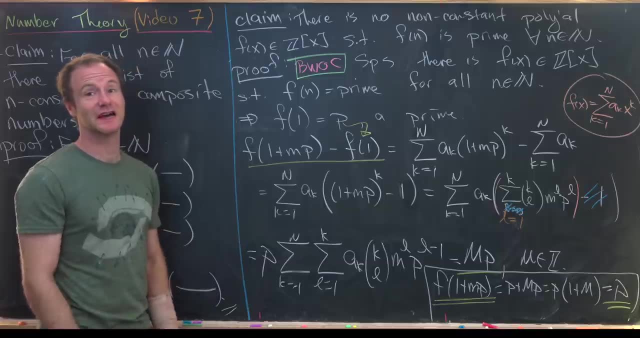 the start, but that contradicts our assumption up here that this is a non-constant polynomial. Okay, now that we've gotten this taken care of, we're going to look at some special types of primes. Okay, for our next little result, we're going to look at something called that Fermat prime. 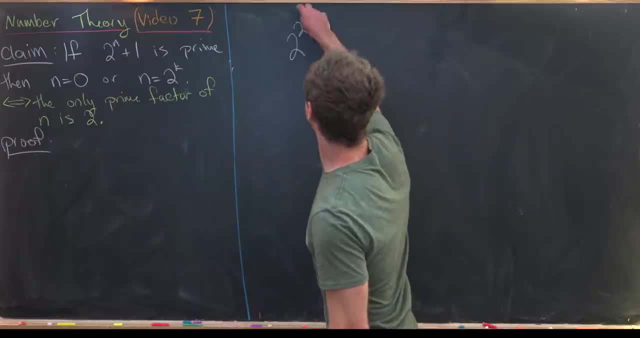 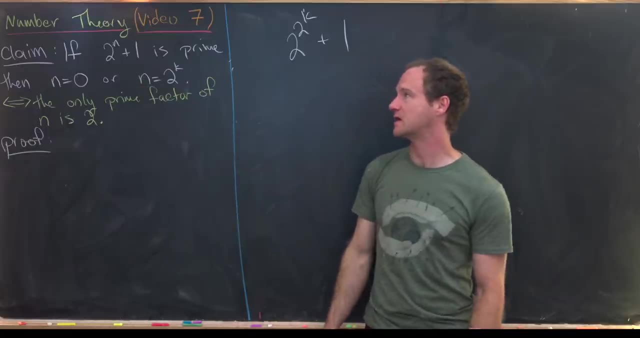 And Fermat primes are of the form 2 to the 2 to the k plus 1.. And what we'll prove is that if 2 to the n plus 1 is prime, then that means either n is equal to 0 or n is a power of 2.. But n being a, 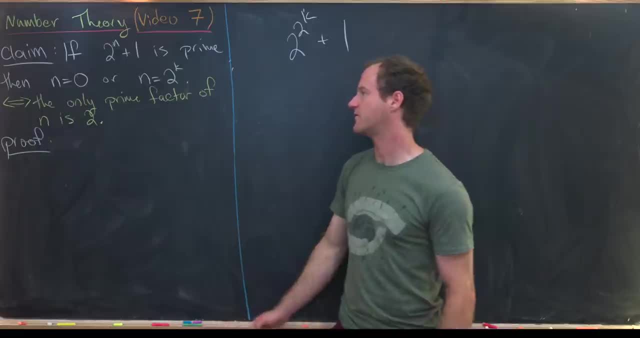 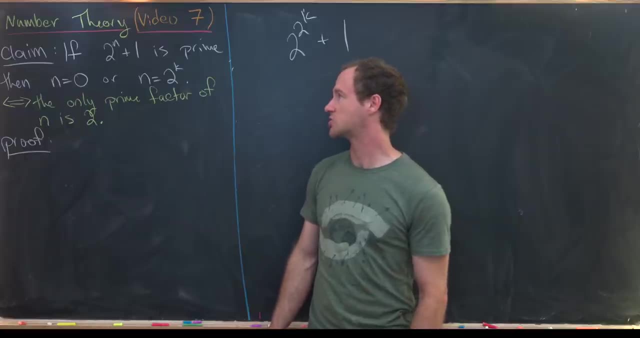 power of 2 is equivalent to showing that the only prime factor of n is the number 2.. Okay, so let's get to this. So we're going to prove this via a contrapositive. So, in other words, we're going to assume that n is not a power of 2, and we'll 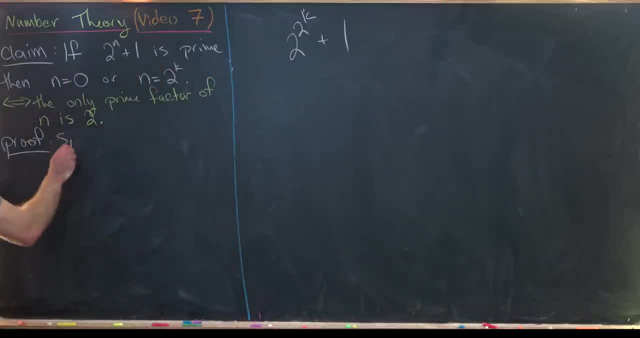 show that this object is composite. So let's suppose that p divides n and p is equal to some odd prime. Okay, but if p divides n, that means we can write n as m times p. But now let's look at 2 to the n plus 1,. 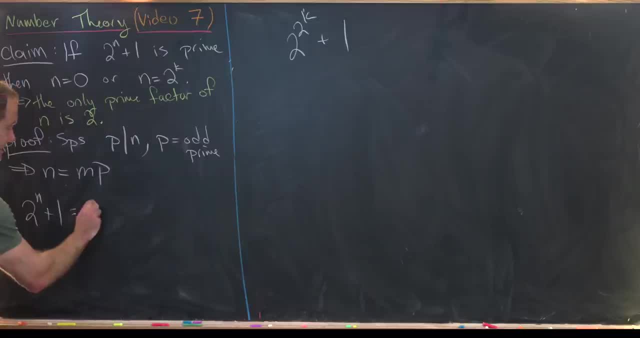 which can now be written as 2 to the m to the p plus 1.. But this has a standard factorization And maybe just think about the factorization of the following: object: x to the odd number plus 1 will factor as x plus 1 times a bunch of other stuff. So just replacing x with 2 to the m, that means we. 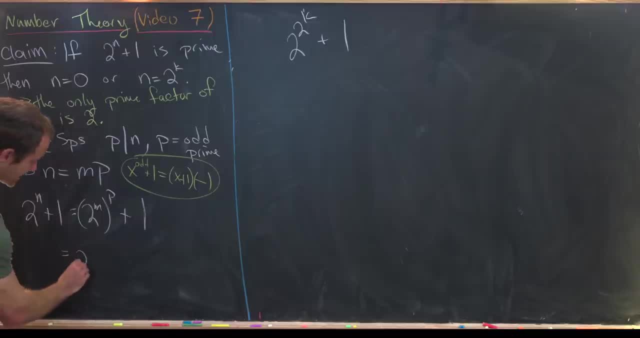 can make this factorization. This is going to factor like: 2 to the m plus 1 times 2 to the m times p minus 1 minus 2 to the m times p minus 2, all the way down to plus or minus 1, kind of depending on the parity of m, And that's going to extend all the way. 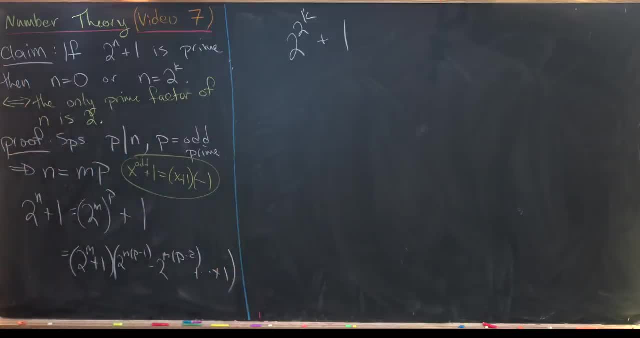 down to just plus 1.. So notice that this is most definitely composite, because it's been written as some number which I'll say right here is a, which is bigger than 1.. And then some number which I'll say right here is b. 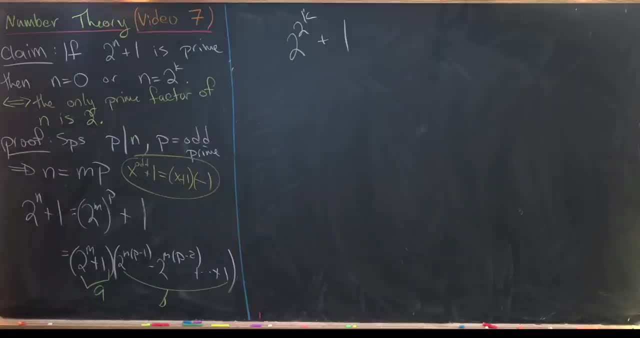 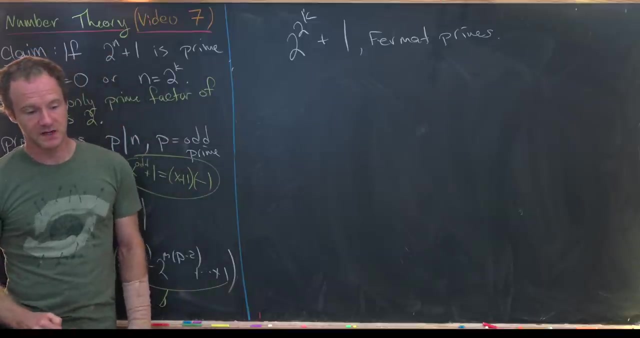 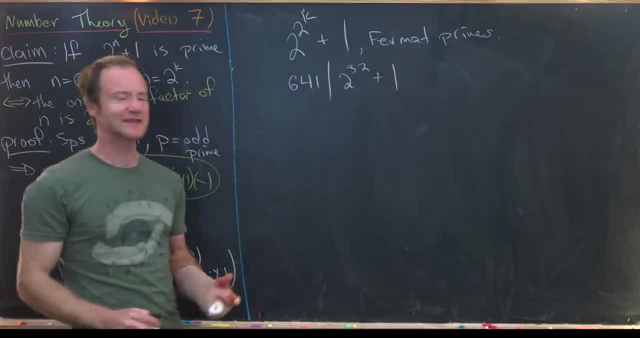 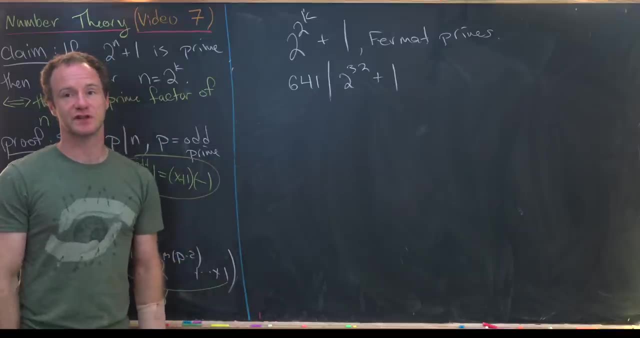 be 2 to the 32 plus 1.. But I guess I should say that 2 to the 32 plus 1 is not equal to 641.. So that'll mean that 2 to the 32 plus 1 is not prime. OK, so we've got one more claim to prove. 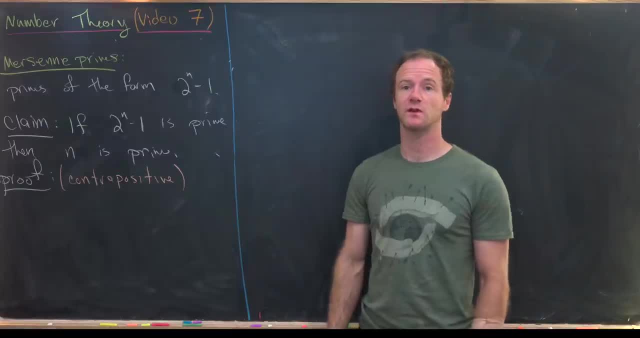 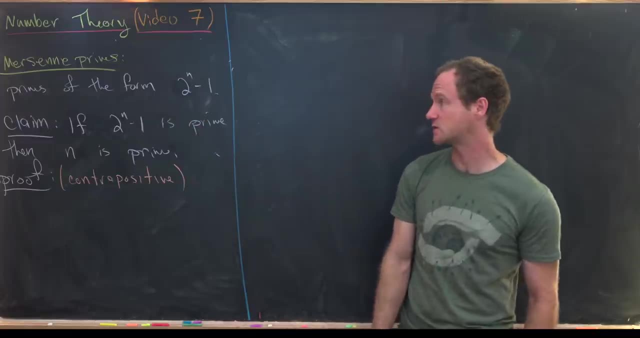 that involves special types of primes. So our next result will involve Mersenne primes. This is a very famous family of prime numbers And they are of the form 2 to the n minus 1.. We're going to prove the following claim: If 2 to the n minus 1 is not prime, then 2 to the n minus 1 is not prime. 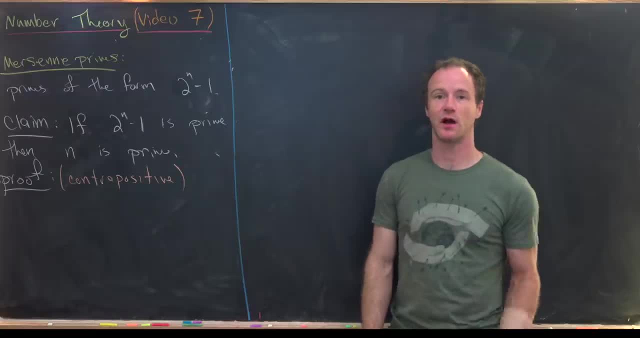 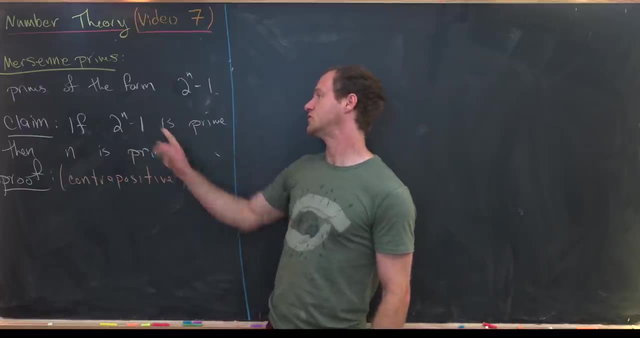 If 2 to the n minus 1 is prime, then n is prime, And we'll do that by the contrapositive. So the contrapositive reads: if n is composite, then 2 to the n minus 1 is also composite. OK, so let's. 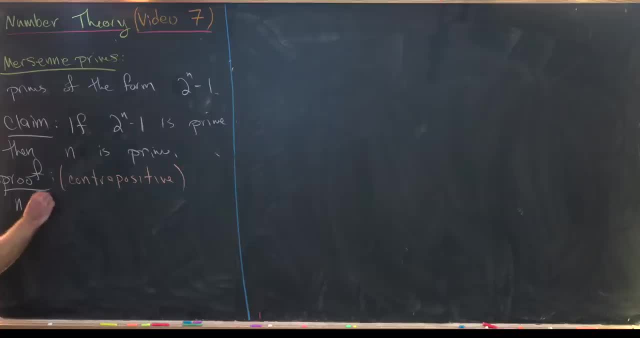 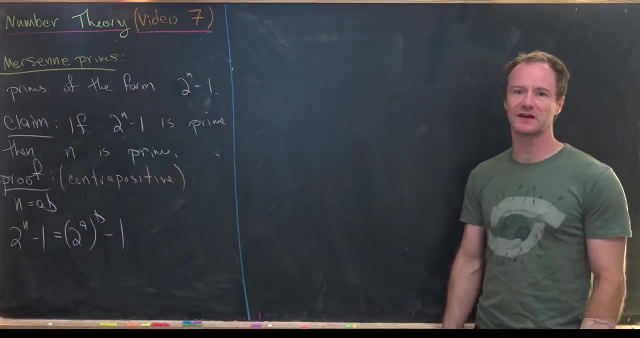 maybe get to it. So let's write n as a times b, And then we can consider 2 to the n minus 1, which is 2 to the a to the power b minus 1.. And we can use a similar factorization formula that we saw before. So this is going to factor. 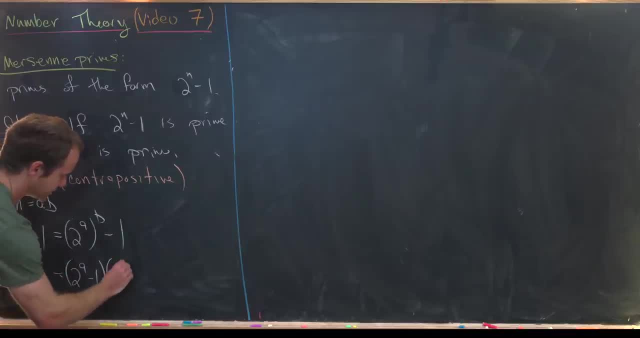 like 2 to the a minus 1, and then 2 to the a times b minus 1, plus 2 to the a times b minus 2, all the way down to 1.. So that proves that 2 to the n minus 1 is composite. That finishes the proof. 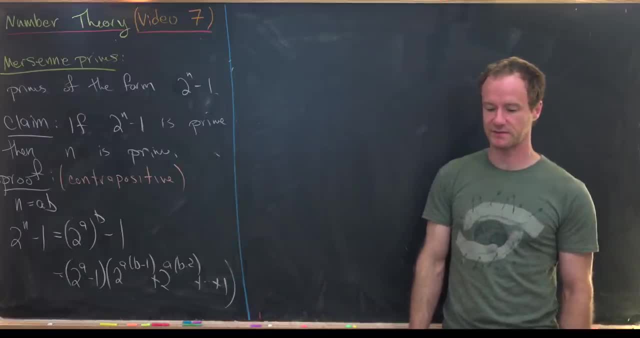 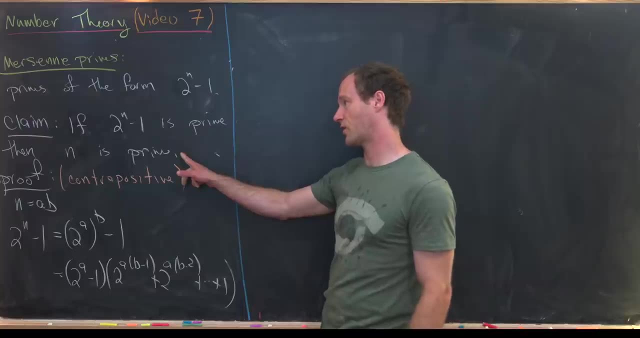 of this claim again via the contrapositive, And next we'll notice that the converse of this claim is not true. In other words, it's possible to have a prime n- we'll call it p- such that 2. 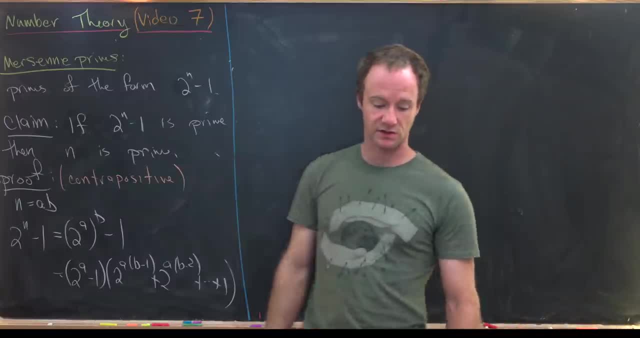 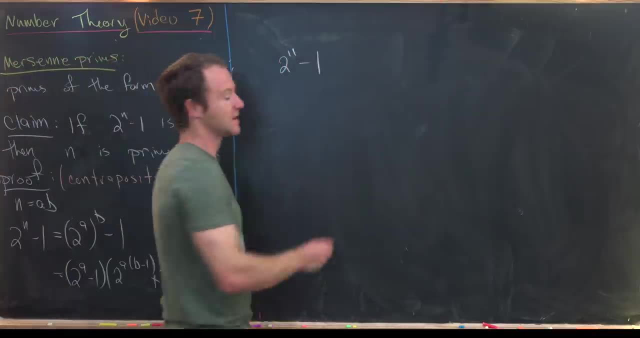 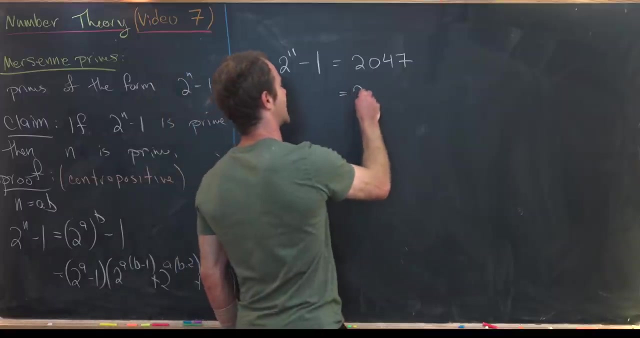 to the p minus 1 is not prime. So let's look at our example. So 2 to the 11 minus 1.. Well, 11 is most definitely a prime, But this is equal to 2,047.. But 2,047 factors like 23 times 89,. 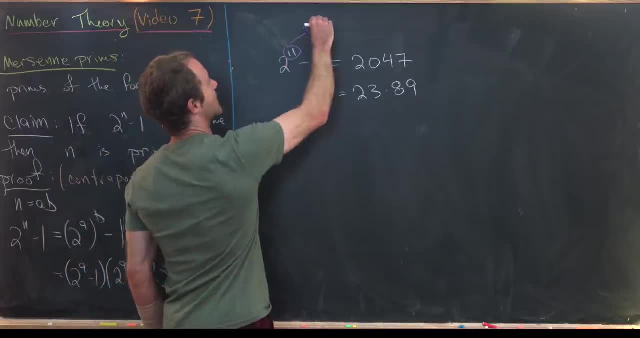 which is 2 to the p minus 1.. So 2 to the p minus 1 is not prime. So 2 to the p minus 1 is not prime, Which means we've got an example where this thing is prime but this thing is composite. 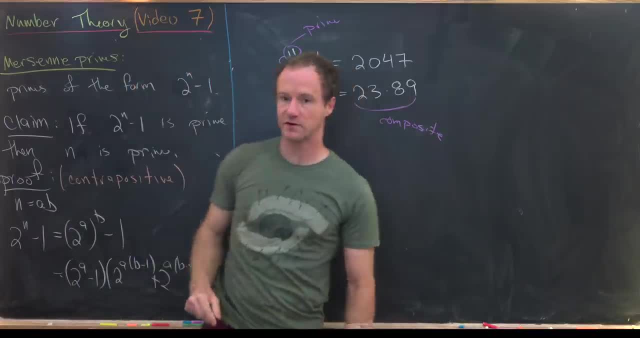 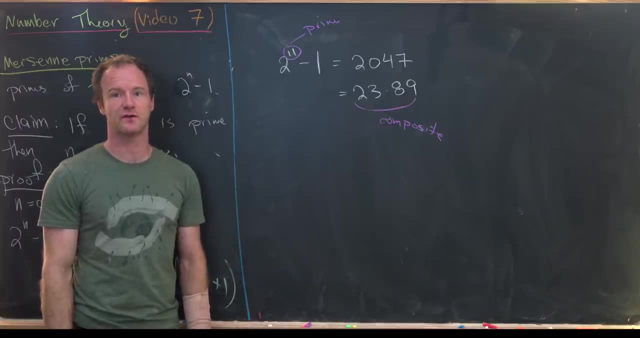 Again giving a counterexample for the converse of this claim. Okay, so we're going to finish this video off with looking at some very famous conjectures involving primes. Okay, now we're going to look at a couple of famous conjectures involving primes. 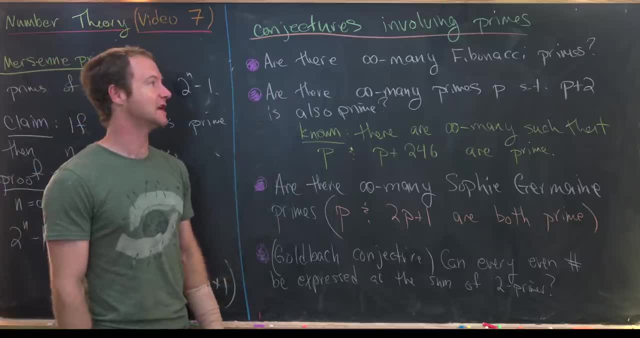 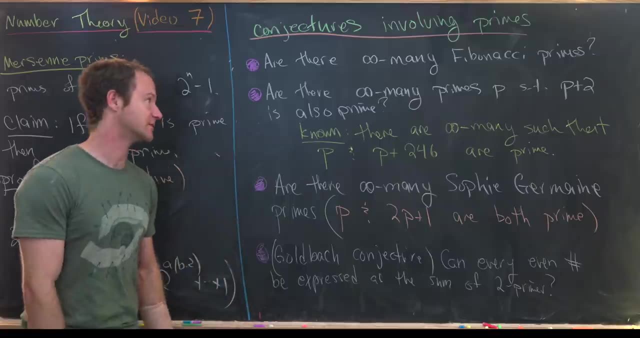 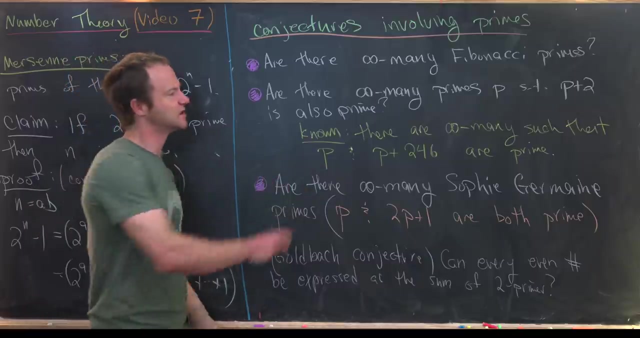 So the first is: are there infinitely many Fibonacci primes? So what I mean is that are there infinitely many primes that are also Fibonacci numbers? Next, are there infinitely many primes p, such that p plus 2 is also prime. So these would be called twin primes, And this is famously known as the twin prime conjecture. 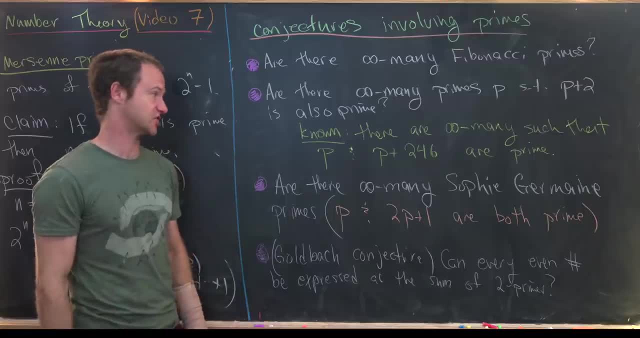 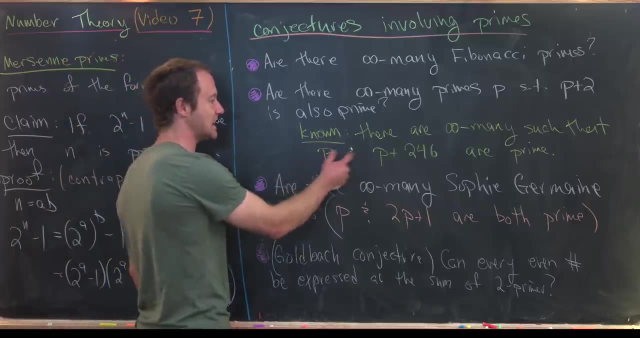 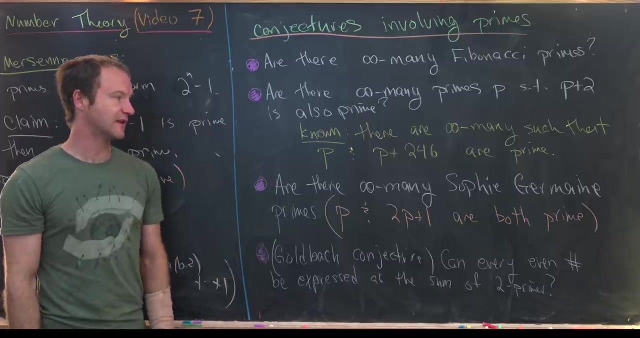 There's recently been a lot of activity towards this conjecture, And at this point it is known that there are infinitely many primes, such that p and p plus 246 are both primes. Next, are there infinitely many Sophie Germain primes, and so those. 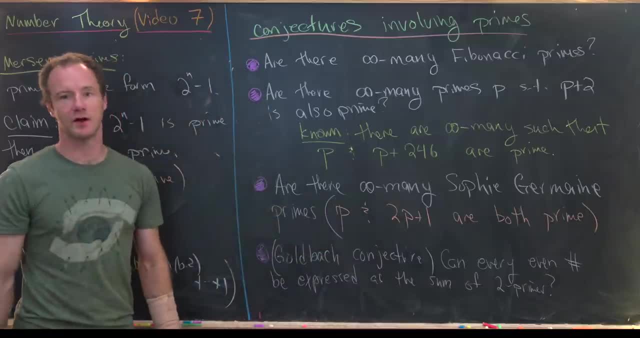 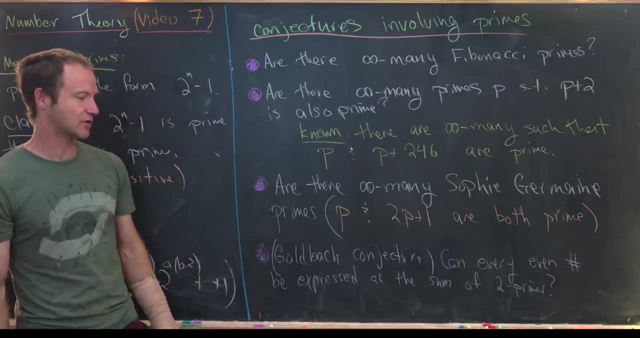 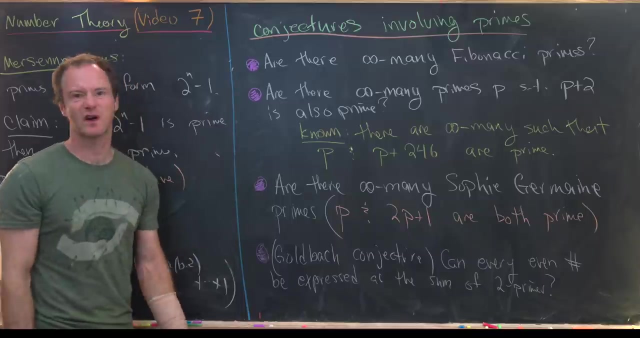 are primes p, where 2p plus 1 is also prime. Then finally the Goldbach conjecture, and that is: can every even number be expressed as the sum of two primes? So obviously this is not an exhaustive list of conjectures about primes, but these are four that are kind of easy to understand at this. 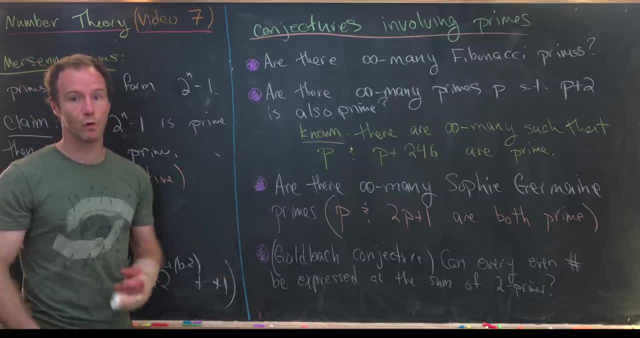 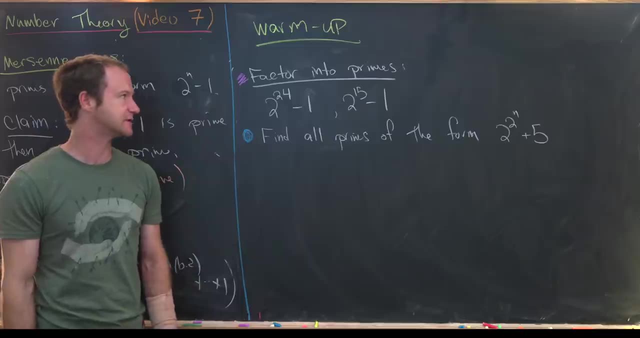 stage in the game. Okay, let's get rid of this and then we'll look at some warm-up problems. So we're going to end with a couple of warm-up problems, and these are built off of some of the tricks that were used in the proofs of this video. So first, factor the following two numbers into: 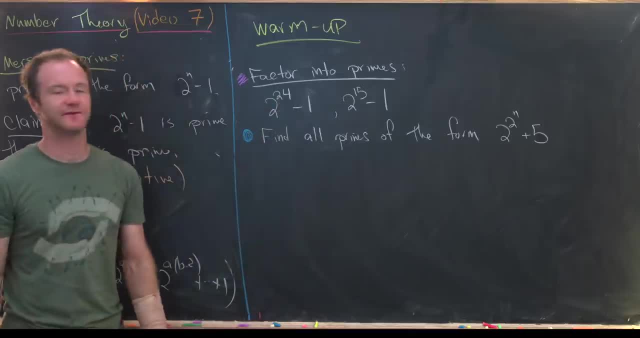 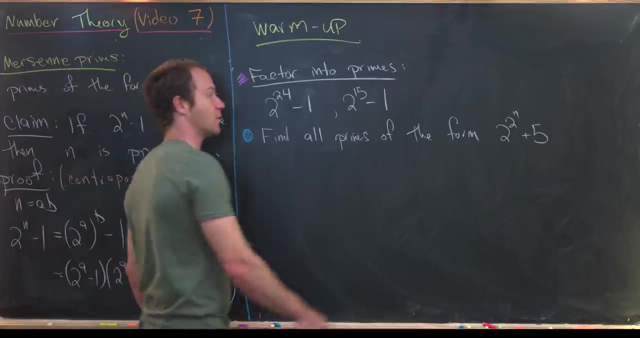 primes, So 2 to the 24 minus 1 and 2 to the 15 minus 1.. So, again, like I said, that factorization, or those factorizations will use factorization tricks that we had in some of the proofs. Then next, find all primes of the form 2 to the 2 to the n plus 5.. So, since the question is to find, 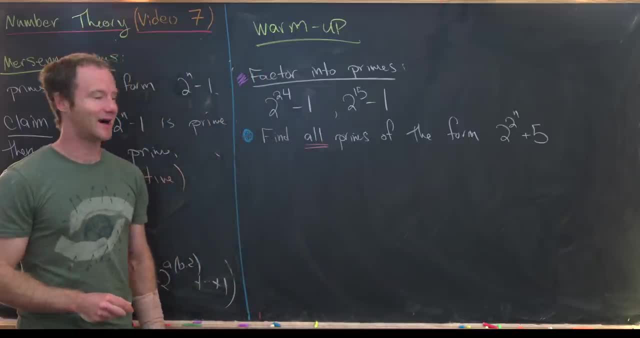 all primes of this form. there's probably some obvious reason why. for sufficiently large values of n, you know no longer get primes. So what I would do is I would make a list of numbers of this form and then notice that that list is no longer prime after a certain point. 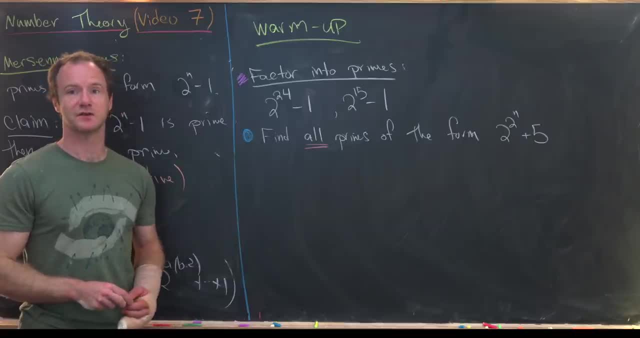 and then let that motivate your proof. Okay, that's a good place to stop.